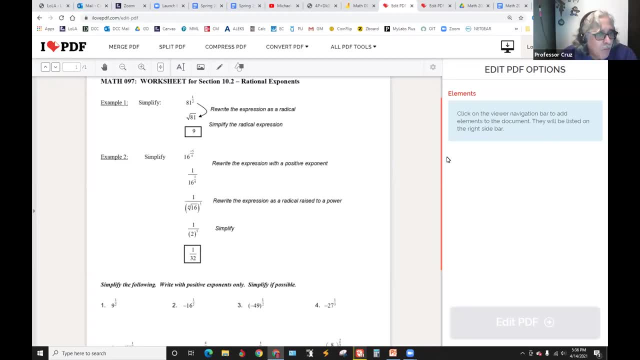 Well, what we have here is our next lesson, And we looked at these examples last time, I believe, but let's go through them again. All right, we have 81 to the power of one half. Now, as you recall, there's a couple of rules we need to pay attention to here. 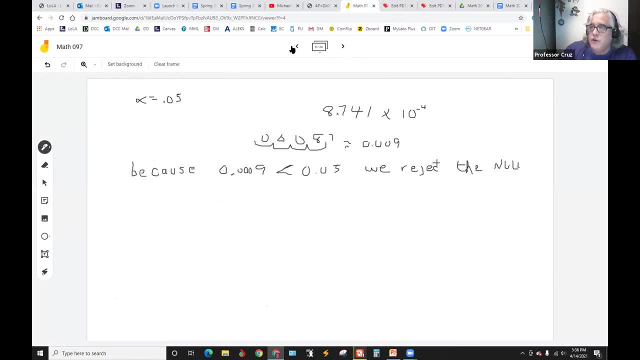 One is an old one and the top one is a new one, since we've been using Okay, this is a fractional rule, So when we have a fraction as an exponent, the numerator and the denominator play a different function. The denominator becomes the index. 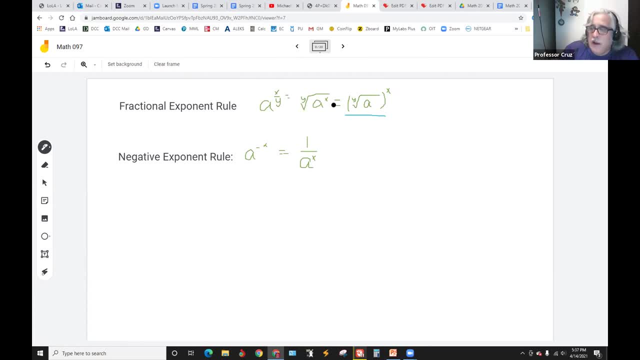 for the radical And then the x. the numerator can appear either on the inside or the outside, depending on where it helps you. For the most part, these are the ones that we're going to do, Because if we do this, blow this thing up first body. 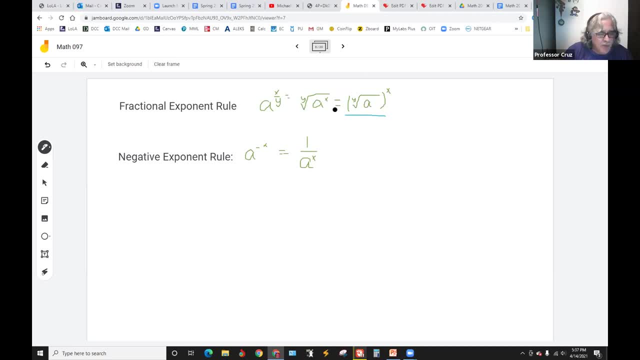 by taking the exponent, it'll be a really big number and then you have to bring it down. This right here, when you take the root, makes it small And then when you raise it to four, it to that power. we'll be able to take that root. There's one case where this might work. 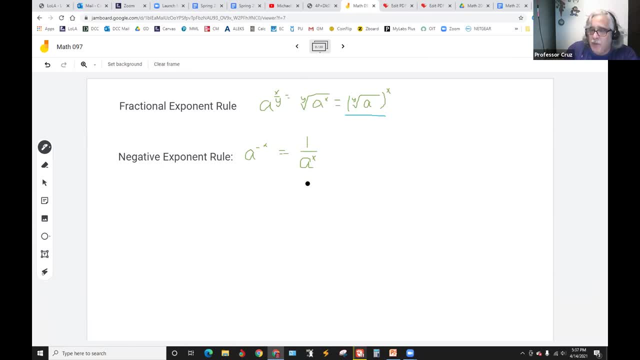 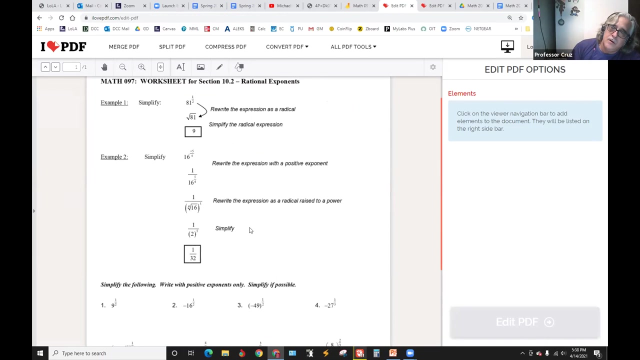 and it'll be towards the end. And just remember the same rule we had before, that a negative exponent means take the reciprocal. Take the reciprocal, All right. so let's go back over here, All right. so 1 over 2, the exponent action, the denominator is 2, so that means we have a square. 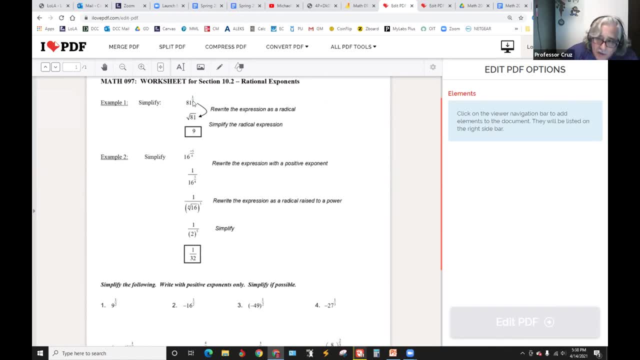 root. The square root is the one without anything crook. It means that there are two inside of there. So the square root of 81 is 9, so this one's pretty cut and dry. Any questions on that? The denominator tells you what root to take. 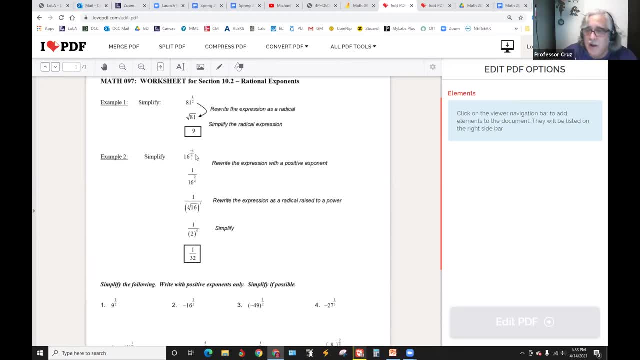 Now example 2, it's a 16 to the negative 5 fourths. So it's negative. so we have to take the reciprocal. That's always the best thing to do first, in my opinion. There might be another way around it, but I would always suggest taking that. 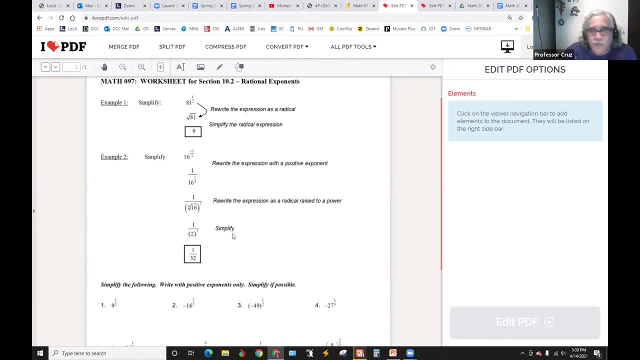 reciprocal first. All right, so we use up the negative by taking the reciprocal. so 16 over 1 becomes 1 over 16 to the 5 fourths. All right, now we're going to use the denominator, the quarter, for a fourth root of that base of 16.. 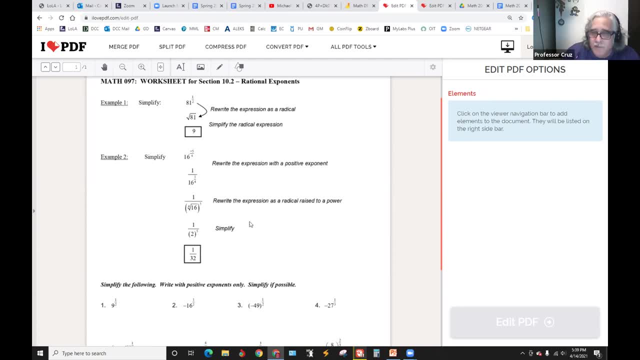 All right, and then the 5 goes on the outside. Technically, we could put the 16 to the 5th power the inside, but that's going to be a really, really, really huge number. I would rather not. 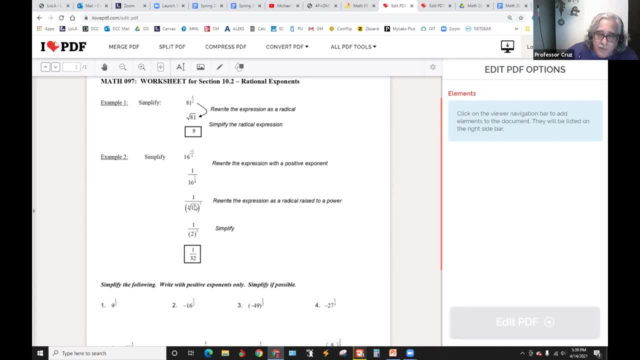 go that direction. so that's why I want to go ahead and take the fourth root of 16 first. So fourth root of 16 is 2.. 2 times 2 times 2 times 2 is 16.. That's why the fourth root of 16 is 2.. Then we raise it to: 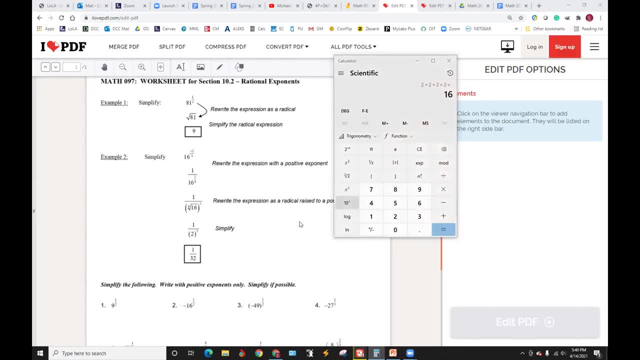 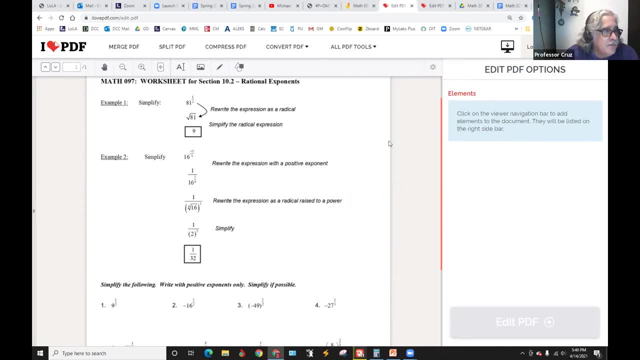 All right, questions All right, and those questions have passed. Okay. so let's go on now to these problems here. The first couple ones are more or less following example 1.. So for example 1,, this has four components, and for example 3,. 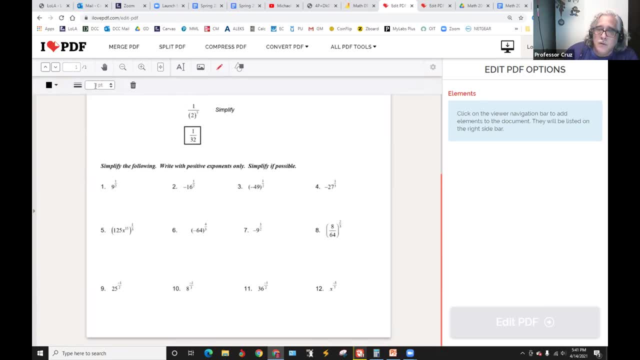 this has n plus i, So this might be said in the process. all right, so 9 to the 1 half power. so what kind of route are we going to use here? it's a square root, so that's a square root of 9, which is 3. 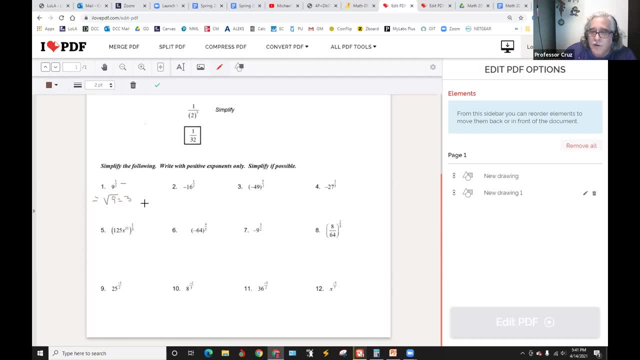 okay, all right now realize there's a difference between 2 and 3 here. so we got to make sure we understand that. we talked a little about this. I think it's in chapter 2. whatever the exponent is touching is the base, so in this case the 1 half is only touching the. 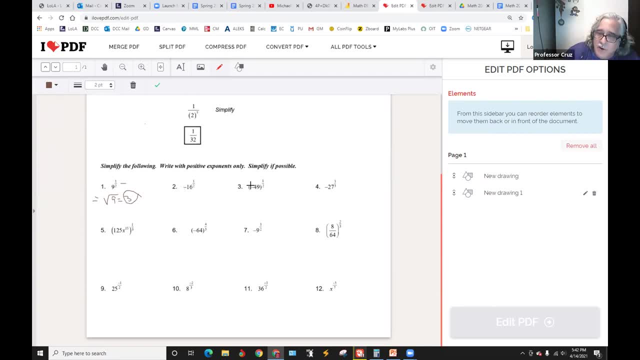 16th. If we wanted to include the negative sign, we have to do what's done here, which is use parentheses to mean that it's going to be more than just the number that's touching there. So the parentheses opening up gives us a negative 49 to the one half power. 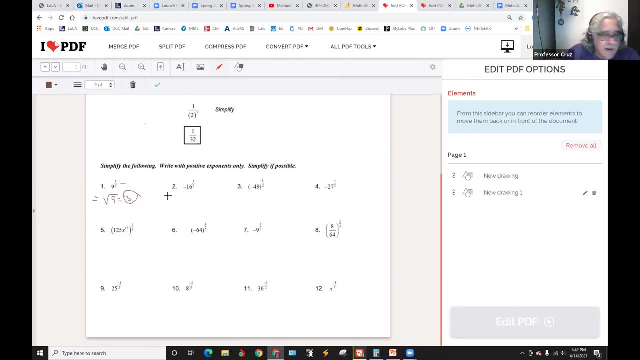 So keep that in mind. Essentially, what number two is saying is: we're taking the negative square root of 16. So this one's another square root and it's going to be negative. All right, look at that and make sure you. 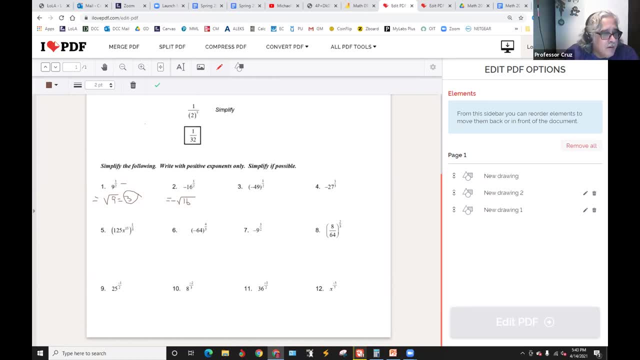 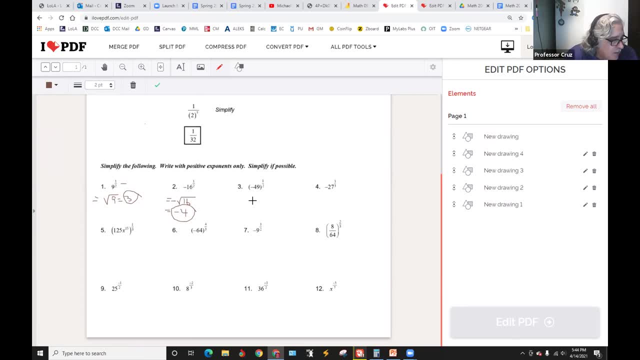 We're the two in the denominator, so Negative 49 is going to be inside. It's going to be what On the inside? Yeah, that's correct. Now here's where we have to think a little bit, because it's going to be easy to jump to a conclusion here. 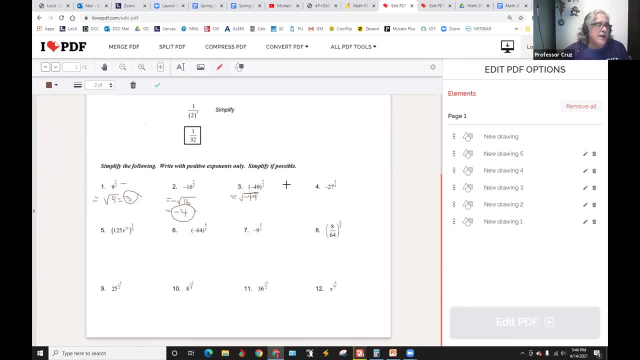 There's no square root, that's negative. Yeah, that's the issue, because a square root means something that, multiplied by itself, gets us to that inside. All right, All right. so there's no way, with what we know so far at least, to multiply a number by itself and get a negative: 49.. 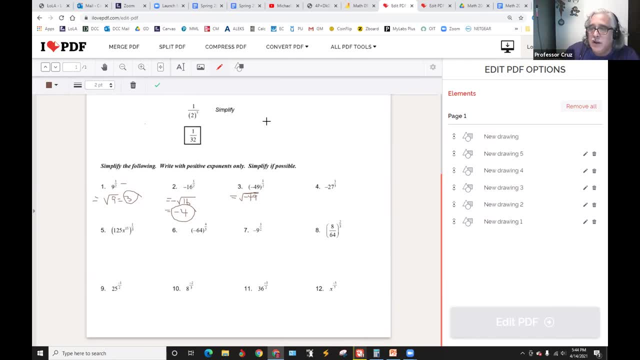 You can try it if you wanted to. First of all, seven squared is seven times seven, which is equal to 49. And then if you take negative seven, That's going to be negative seven times negative seven, which is also 49.. 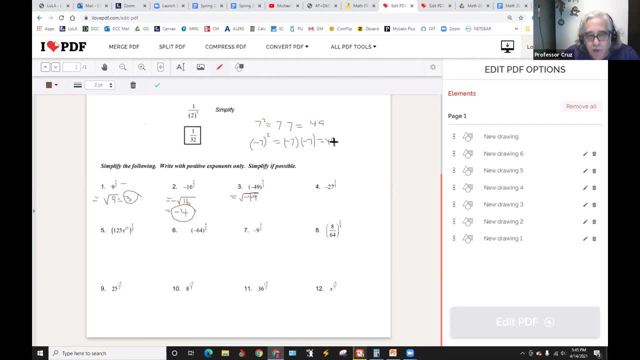 So one thing that we can rely on is the square root of any real number. I'm sorry, the square of any real number is going to be positive. Now, the key word here is real number. Now remember back in the first chapter, where we talked about the different kinds of numbering. 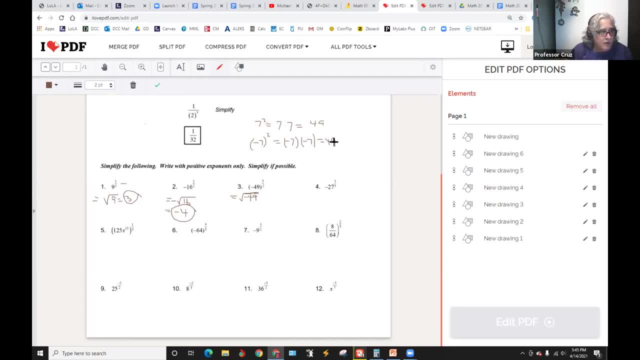 You started out with the bottom. You have natural numbers, which are the counting numbers, Then you go to whole numbers, which is zero, And then you go to positive and negative, which are integers, And then you go on to rational numbers, which are numbers that can be expressed as a fraction. 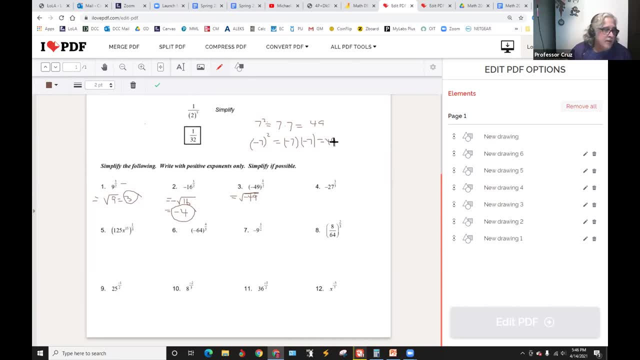 which includes all those numbers at the bottom, because even a whole number can be expressed as a fraction by putting it over one. Now, as we work our way up, we've got the numbers that we're talking about in 7.2,. 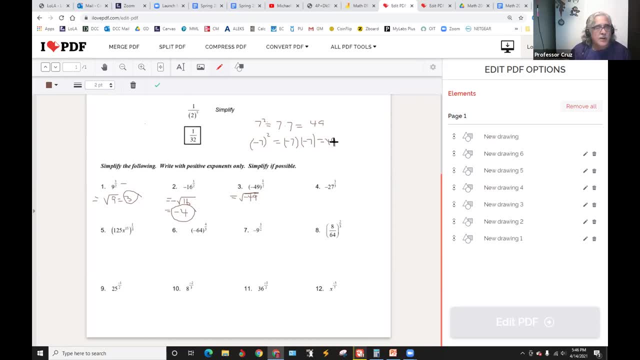 which was something like square root of two or square root of three, which cannot be expressed as a fraction because they're repeating decimal. All right, So we're kind of at the top of the food chain And in the end of this chapter. 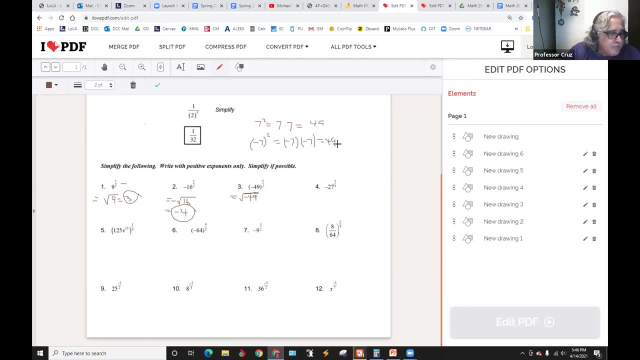 we're going to find out what this is called, But for right now we're just going to say not a real number. All right, Not a real number, And that doesn't mean those terms being slightly something different. They would, in kind of common language, like real means that it exists. 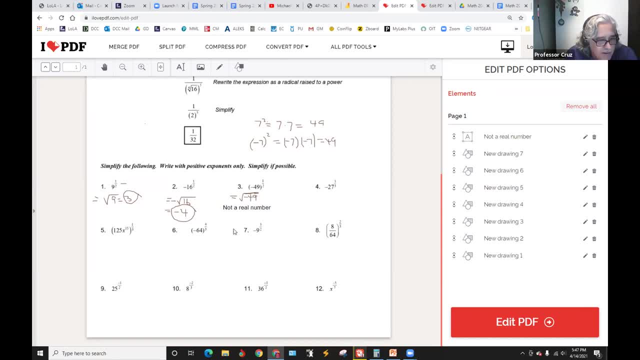 But there's a set of numbers We're going to talk about in 10.7, called complex numbers, And we'll find out that there is a way to evaluate this Now. this one here, this 27, is the base. So 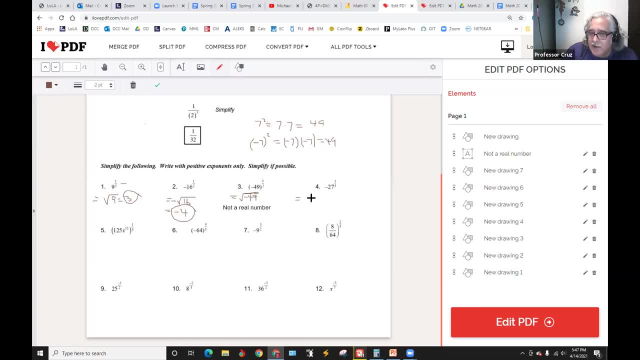 This, though, is not inside the negative. It's not inside, So we're just going to write it as: And that's supposed to be a three, It's a negative three, And that's going to be negative three. Good. 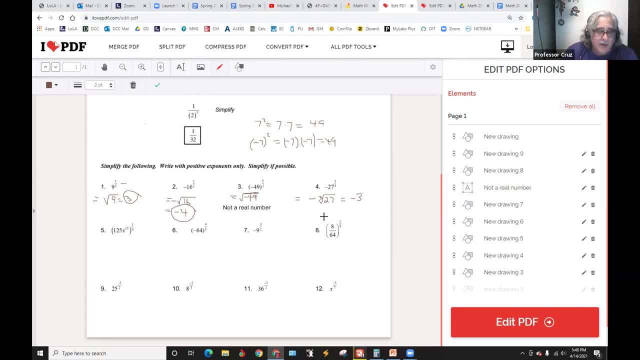 So three times three times three is 27.. And then the negative sign was on the outside, So I'm making sure that this Was going to be negative, Okay, So Let's move on a little bit. Well, here's one more. 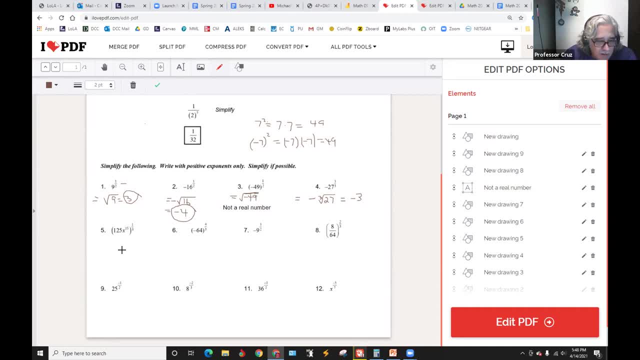 That's got only a one in the denominator, So we don't have to do too much here. but The parentheses mean that all of those things Are inside The. I'll read a story, So we're going to put everything underneath there, and that's another third root. 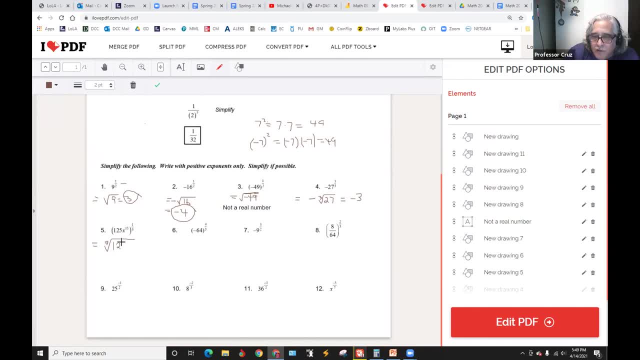 So we've got a 125. X to the 15th And I had somebody in my morning class, another teacher, come to visit and she had informed me that the official calculator, you know the one that looks like this: 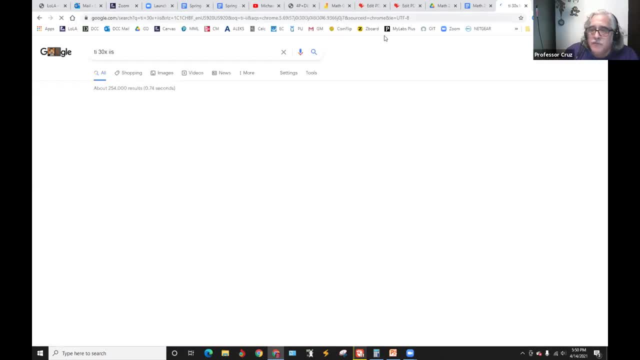 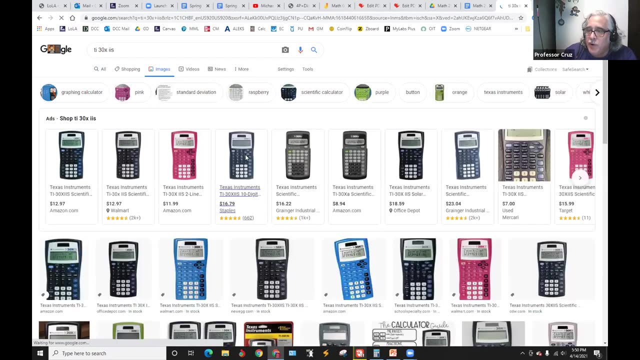 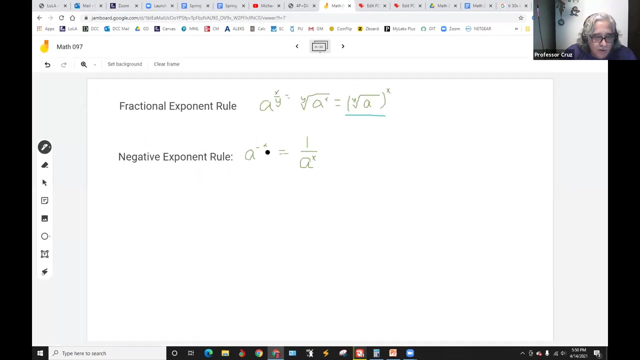 Here. it is The one that's the official calculator for the class. Well, I actually do what I'm trying to show you on here, So you might take advantage of that, because you're free to use that calculator on the exams. Let's see. 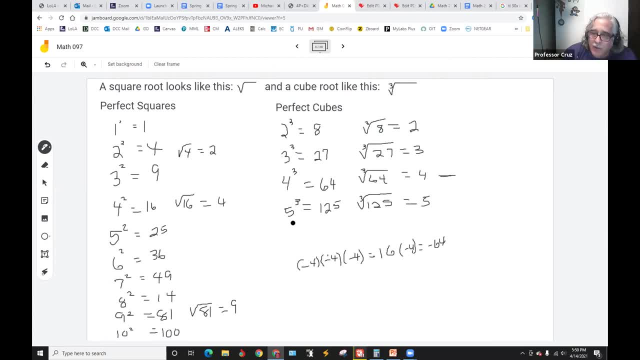 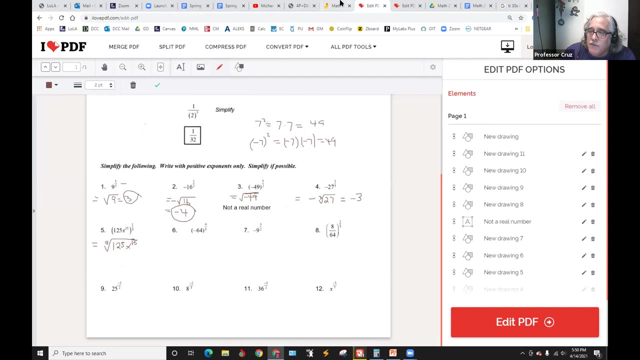 So my way of doing it is just I write these down and then refer back to them, And so the thing we need to be looking for is cube root of 125,, which is the top one here. and that's five, All right. 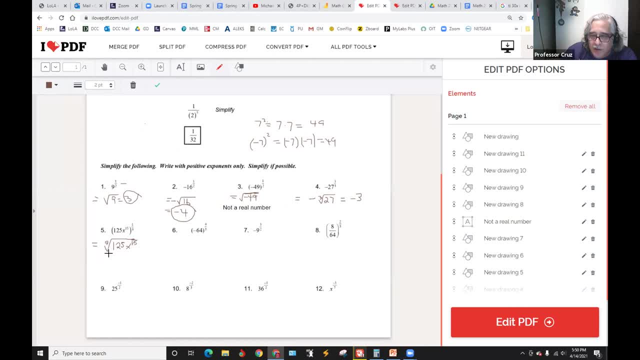 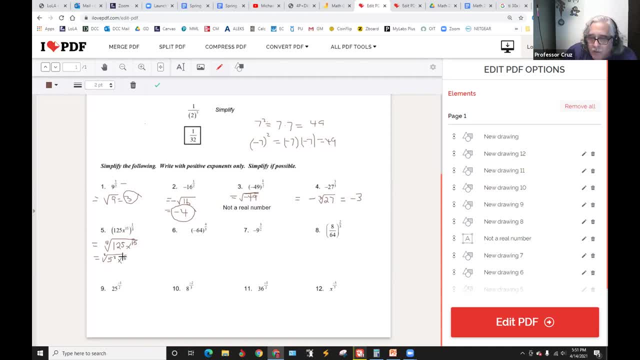 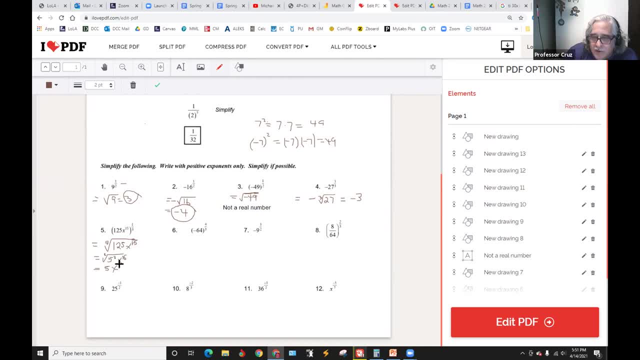 And three into fifteen goes five times. All right, Make sense. Yes, All right, All right, i got on here late and i had a question about number three. okay, go shoot. um, why is it negative 49, not a real number? yeah, it wouldn't. be uh, negative seven. okay, look up here at the top. 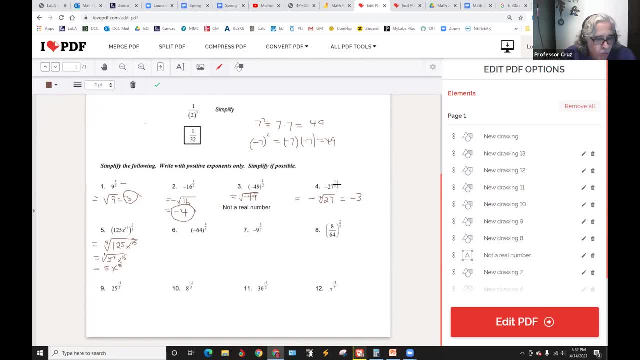 negative. seven squared is what negative seven times negative seven seven. yeah, that's 49. any number that's squared, any real number that's squared, is going to always be positive. okay, negative, because there's two negatives here. negative times negative is a positive 49. so find me the number, the real number. 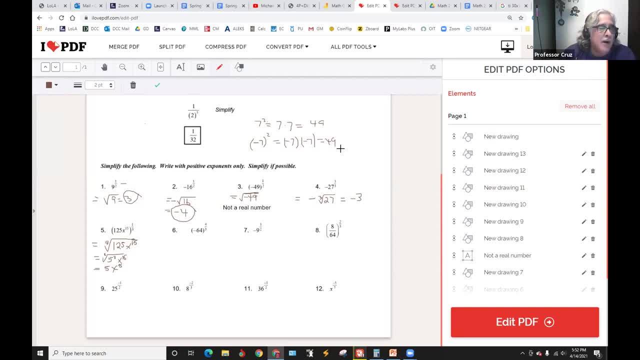 that you can multiply times itself and get positive- i'm sorry, negative- 49. i'm gonna wait here until you find that number for me. i'm gonna wait a long time because i'll just tell you, here there are no numbers that you can square and get a negative value, no real numbers. okay, so that's how it works now in. 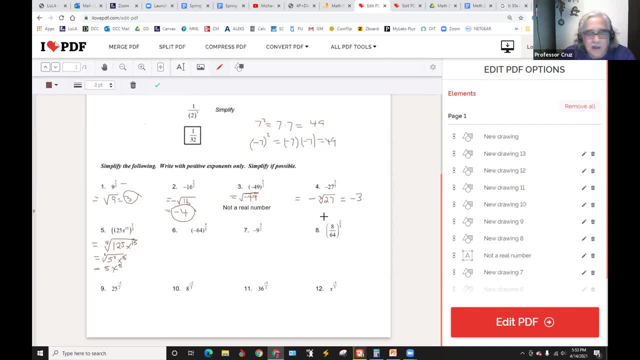 uh, section 10.7 i believe it is. we're going to learn about complex numbers, so we're going to be able to evaluate this further then, but not now. so that's kind of what it amounts to is there's no way to multiply a number by itself, positive or negative, and get a positive real number. 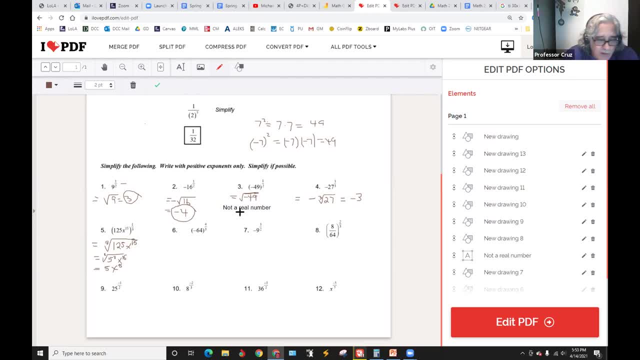 so that's why we're saying, for right now, it's not a real number. that does not mean that it does not exist, because it does, it's just that it's not a real number because you know, thank you. real numbers are the highest form of numbers we know about so far, and we're going to learn about complex numbers. 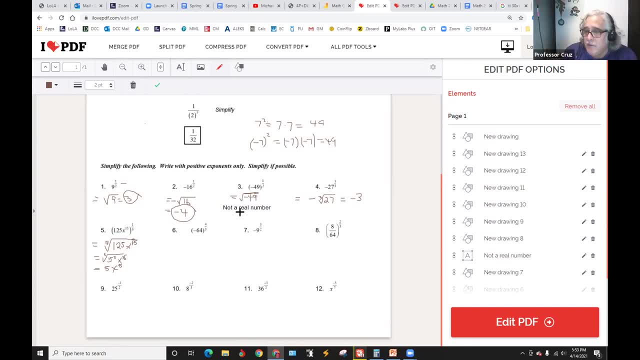 at the end of chapter 11.. i'm sorry, seven. all right, so the next one are all going to have numerator and denominator. so this is a third root down there in the bottom and the whole thing is inside the third root, the negative and the 64. now this is a bit different than this one because it's a new. I'm 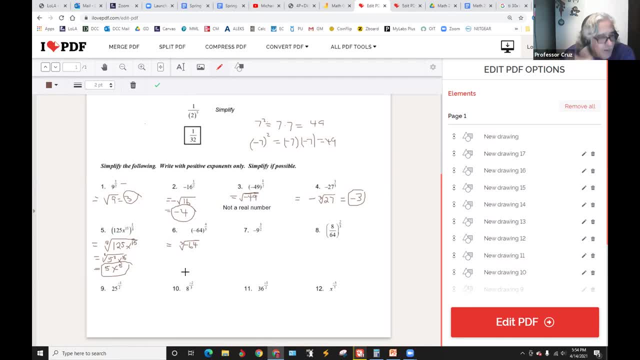 sorry, it's an odd root. you've got three times, you're going to multiply the same number and there are three negative signs. so it's possible to have that negative inside for an odd root like this. for third root, so we can go ahead on this one, because I think we even talked about it the last time. 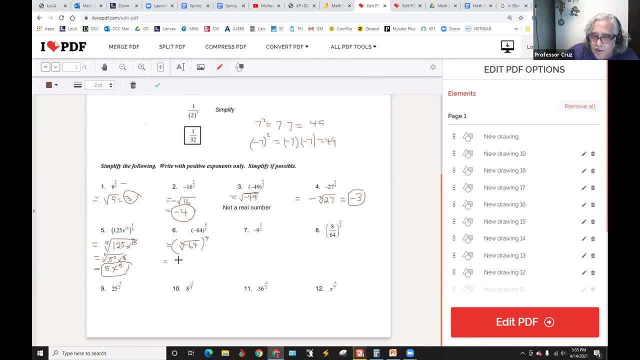 the cube root of negative 64 is negative 4, and then when we take negative a 4 and raise it to the fourth power- negative 256- it's not negative because you got an even number right there, oh, I'm sorry. so it'll be 256 positive, because if you 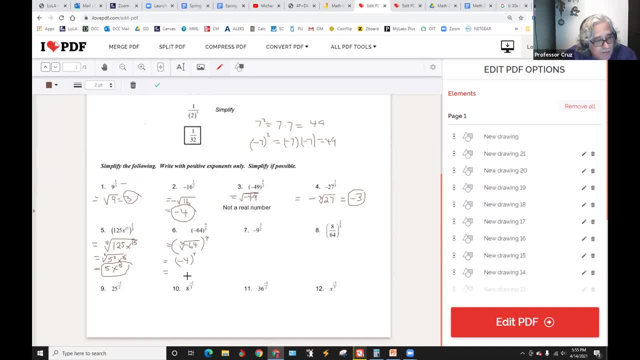 take negative 4 times negative 4, you got 16 positive. the other two four is also giving it a positive 16. you multiply positive 16, that positive 16, you get positive 256. all right, so you still should do that, excuse me. so seven: the base is only the nine. it does not include the negative sign, so 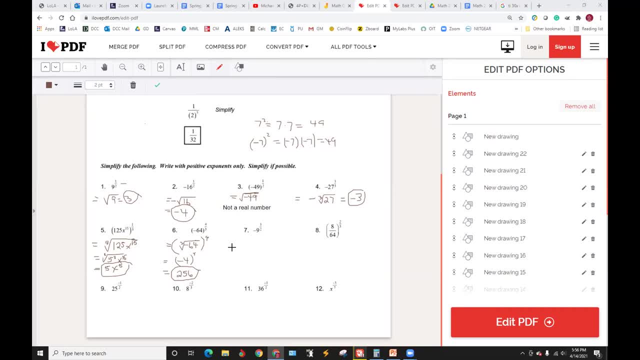 that's why we got to make a distinction between two and three. so this is going to be negative and it's the square root. all right, you don't need to put the two there, but I'm just kind of showing you, and then this whole thing is going to be cubed and again the negative sign is not part of the base. the nine is the. 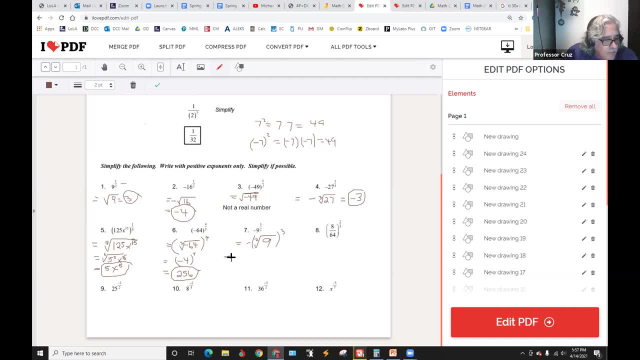 only thing that's in the base, so that's square root of 9- is 3, right, and then the negative sign. this comes along for the ride. so this is negative 27, right? yeah, all right, I'm gonna go this direction to. this proposal needs all the space we could get now. this is the dot. 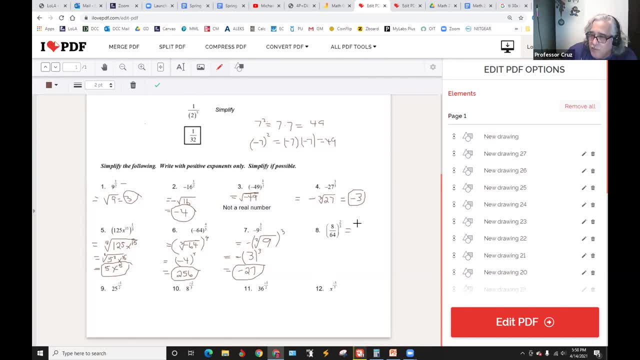 denominator is cubed as a 3, so basically it's a cube root. all right, so C is velitchy and V is three, threes square root of 24 andщее in there it takes that denominator to calculate. it's a fractional cube. its denominator is cube is a together this: 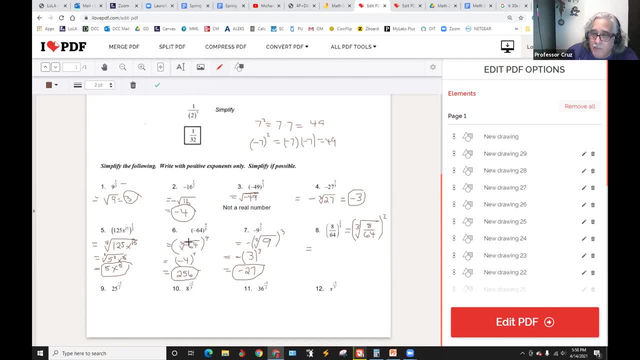 denominator is cube is a three, so it's a cube root and it's got a fraction in there. okay, it's got 8 & 6, 4 is you just put one over the numerator and one over the denominator. if that makes it clear to you, you use that in order to evaluate. 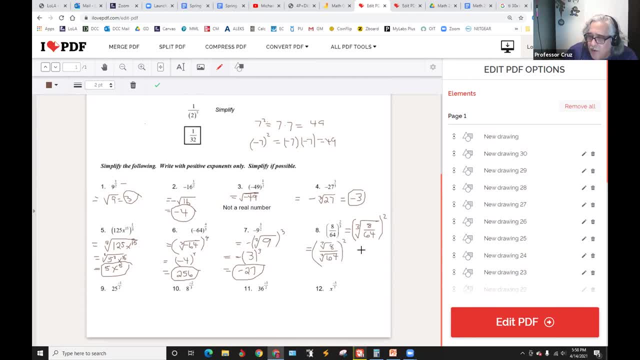 and then we're going to square. so the cube root of 8 is 2, the cube root of 64 is 4 and that's all squared now. all right, it's probably going to be easier if we simplify this now. two fourths is one half. 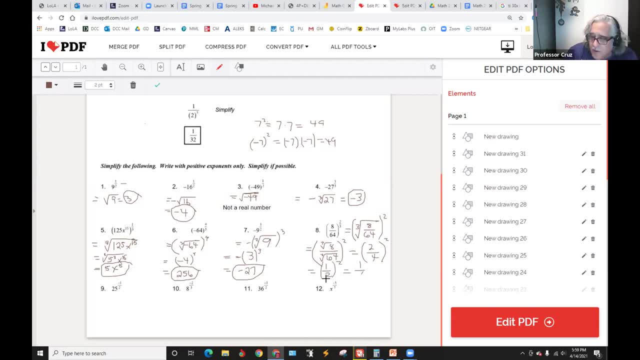 and when you square it it's one. fourth. one times one is one. two times two is four. okay, let me know if you got any questions, because we got plenty of time. hmm, okay. so uh, professor cruz, just for that last one, um, because with 8 and 64 that can already be simplified down. 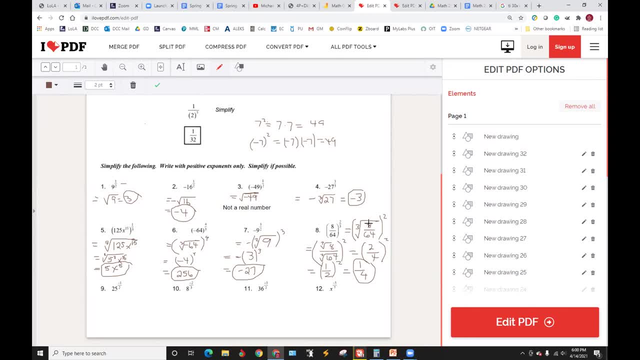 to one eighth. you pretty much end up at the same answer. so does it matter? if you do that, what are you talking about? where, uh, the 864th? because if you minimize 8 or 64, that ends up being one eighth, correct? yeah, you're right. you're right, i mean. 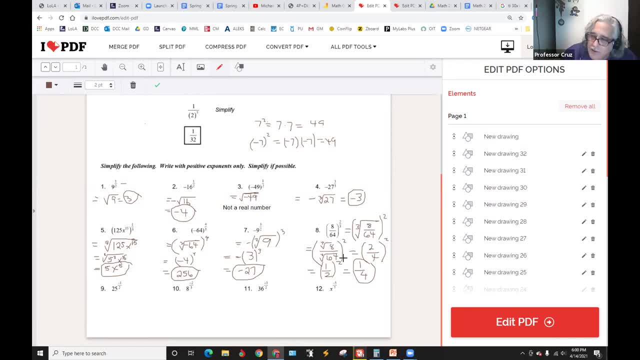 let's see, yeah, and then one, and then the one goes, and then it would be, and then the eight would be two. you're right. you're right. yeah, i never i didn't think about that, but that you could simplify it up there, as long as the fraction is fully inside that same radical, yeah. 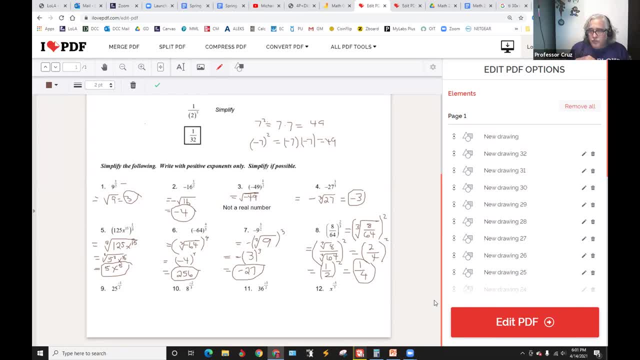 you can do that. okay, i hadn't noticed that. i probably would have made a little bit shorter if i had done that. yeah, i was just asking because that's i ended up with the same answer as you, but i went about it the other way. that's fine. yeah, because in here you can just eight. it goes into eight one time and 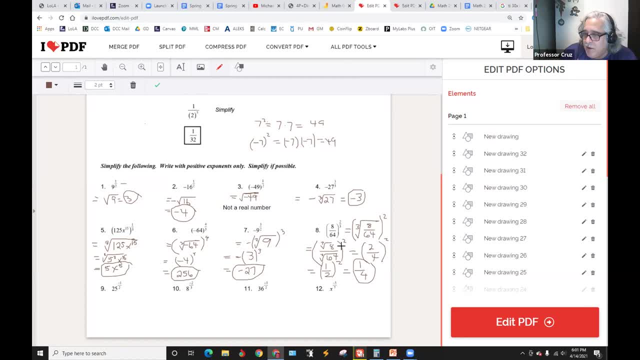 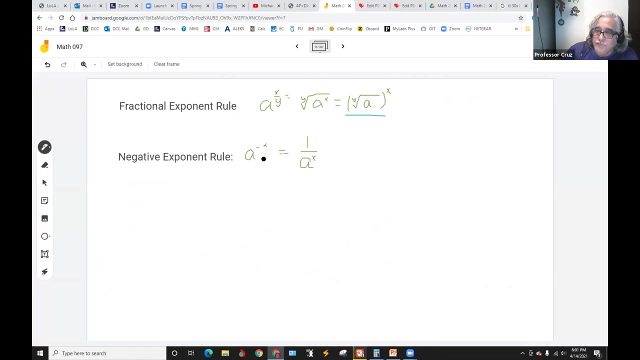 uh, into 64, eight times, and then the cube root of one is course one and the cube root of eight is two. all right, now we're getting into some negative into it and remember, negative means: take the reciprocal. all right, that's the only meaning of negative exponent. 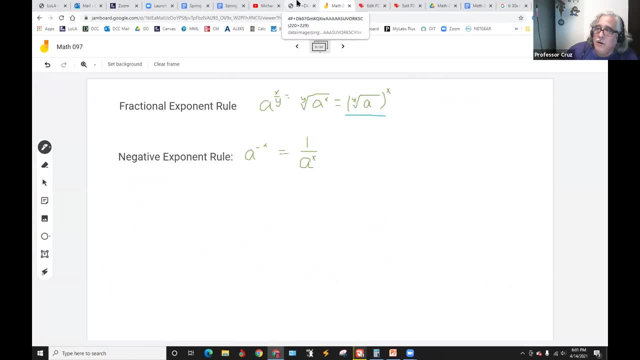 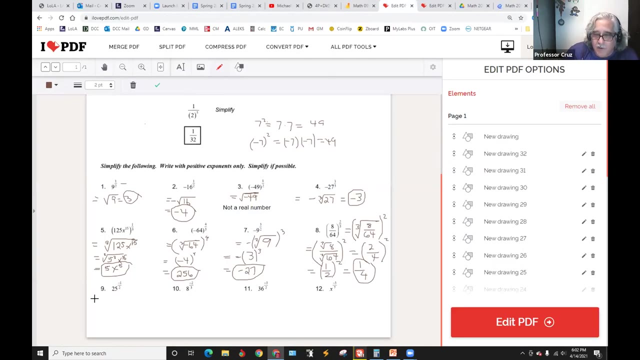 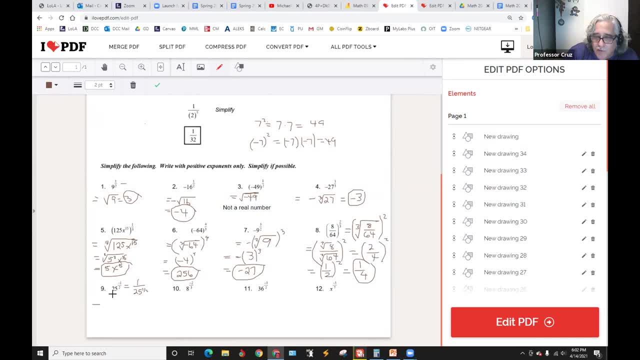 so that's going to be one over the square root, 25. Okay, Well, again, I'll take it for me. You, You, You. Okay, we got another negative one. it's going to be a cube root, but first we take our reciprocal And it's going to be brought up to the power of two-thirds positive now because we took 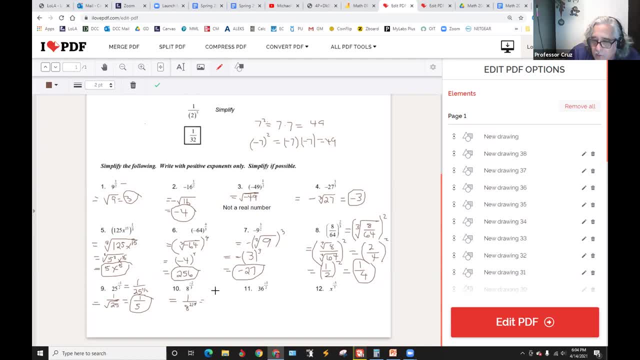 So let's see then that's going to mean 1 over cube root of 8, All square. So the cube root of 8 Is 2, And then what squared is 1 squared quarter. Things turns down to 1 quarter. so check it for me. 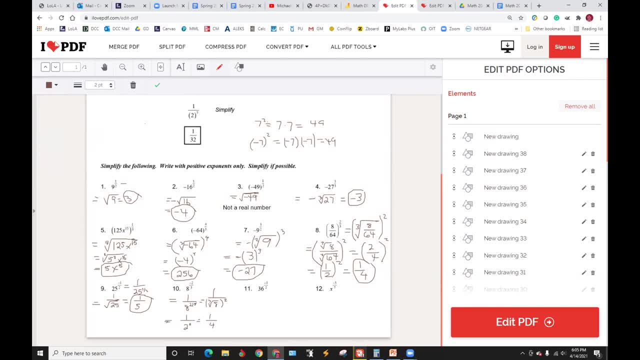 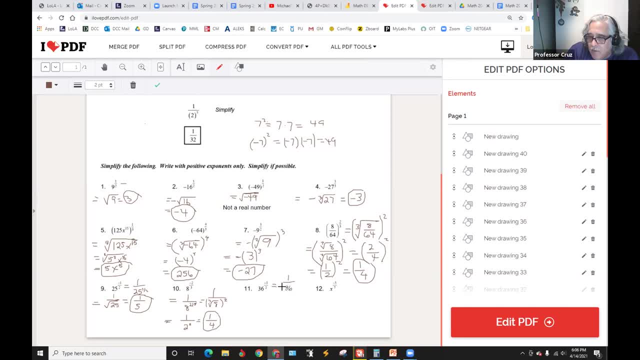 And so we got 1 over 36, And so we got 1 over 36, and So our Plus the number 3 order, plus 3 üzer, plus 3 üzer, So 1 over square root of 36 is 6, and cubed, I think that's 216, right. 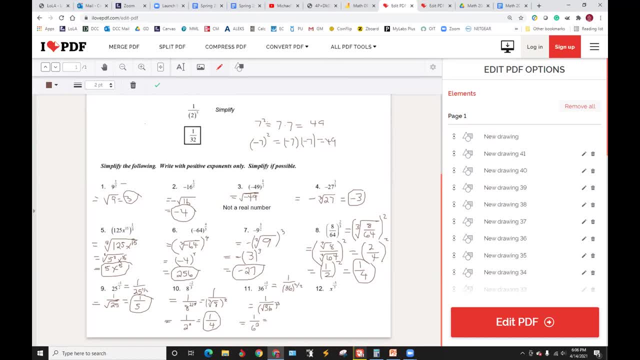 Yeah, 216.. All right, I'm going to go over on the other board and I'm going to write another. this one is kind of strange. I want to find one that's a little bit. I want to make up one that's a little bit better. 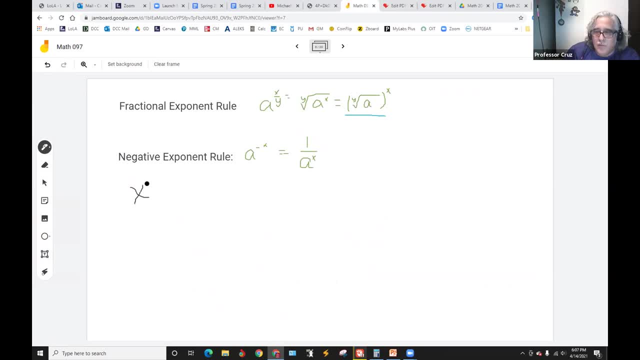 I want to turn them upside down, those numbers, seven-thirds, but it's still going to be a negative. All right, so you can do this with variables. this is the one that's on that sheet. you can do with it, you can work it, but it's nothing really happens. so I'll show you. 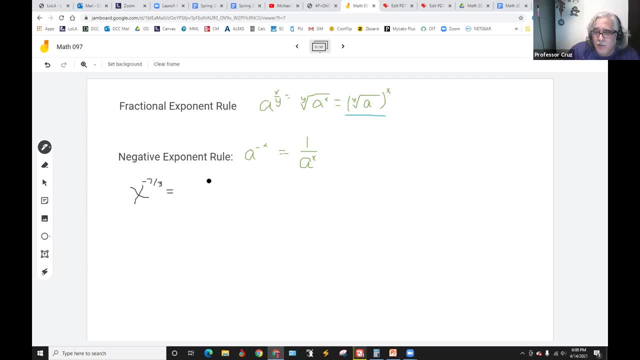 So what we got here? we're going to take 1 over to get rid of our exponent- I'm sorry, our negative sign in the exponent. and then what we got here: the denominator is 3, so that means: 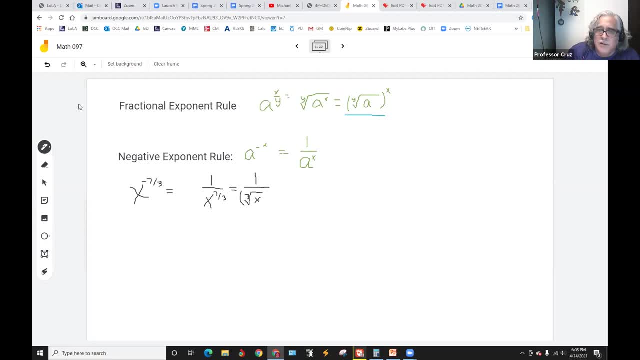 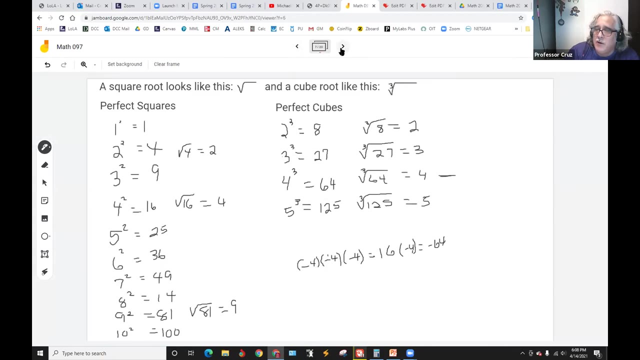 I'll tell you what. let me back off one stop instead of doing what I was gonna do. put it on the outside, like we did with the other ones. I told you that you can put it on the inside of the outside, whichever helps you. well, this one if. 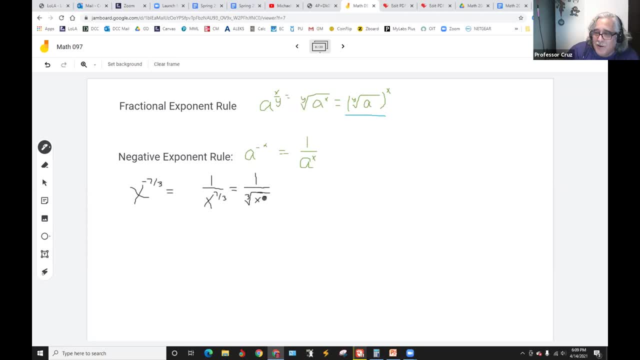 you play it on the inside, it's going to help us a little bit more because these are not numbers. you know you can't really evaluate X to the seven, since we don't know what it is, or the cube root of x, because we don't know what it is. 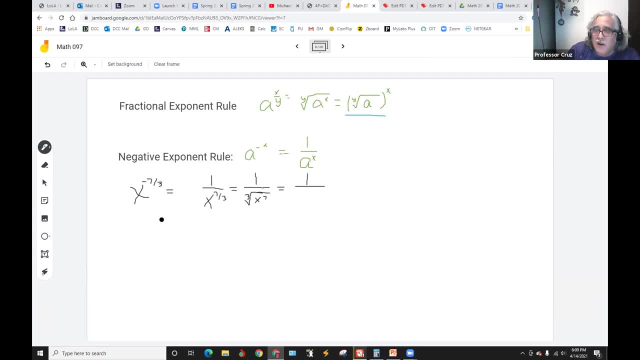 All right, Now we can play the thing that I showed you about taking the index and dividing it into that exponent, and that goes twice, right? Three goes into seven twice. So you got an x to the squared that comes out, but you got one that stays in. 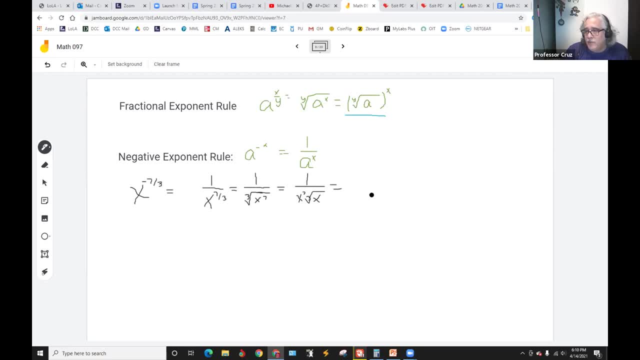 Maybe that's kind of hard to see. Let me rewrite it So that would be the simplified form of it. Right there, That's all you can do On this one over here. why I thought this one was kind of silly. 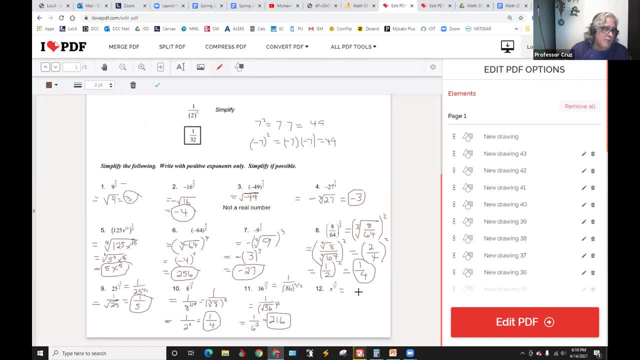 I don't know why, Because these problems they probably come from my math lab And those things are algorithmically generated and probably somebody doesn't check every one of them to see whether it's a good problem- Not that it's bad. 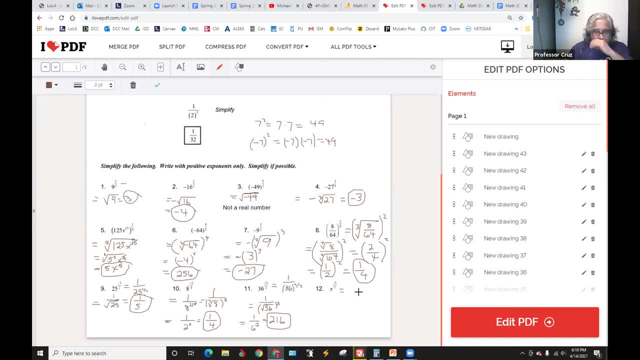 It's just that nothing exciting happens. that proves a point. So what happens here is when we get two, here we three, here we two, here two, all right, So we have one of those zero and one of those zero. 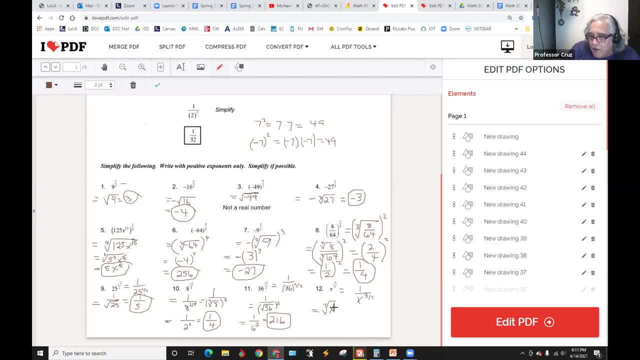 All right. So this is it All right. So this would be the seventh root of x to the third, And nothing can happen there because the index is larger than the power there. So that's all you can do. 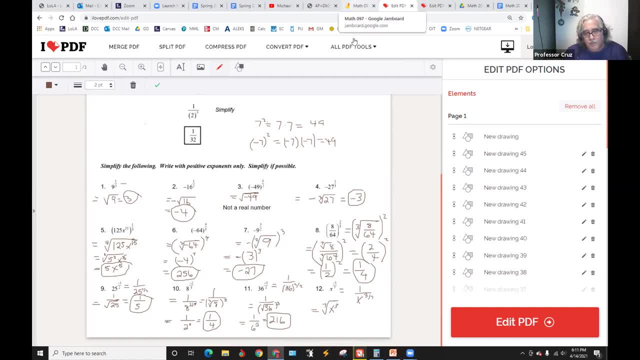 Well, I just wanted to make up one where it actually changed a little bit. All right, Thank you, Professor Cruz. for number 12, it wouldn't be a 7, correction: a 1 over that 7x3?. 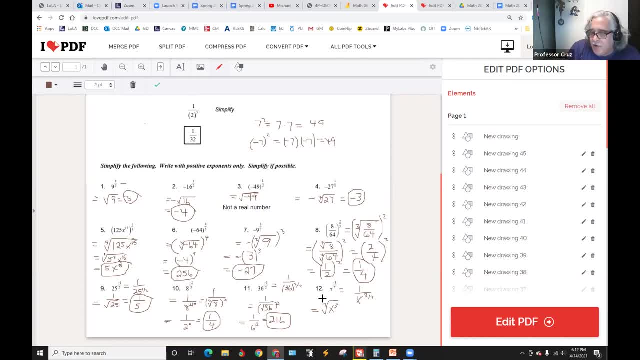 Well, we did it here. Oops, yeah, you're right, Sorry. Yeah, I just forgot to put it. I was trying to write small and I ended up. Okay, Okay so. So that's all we got on this. So any more questions on any of these before we move on? 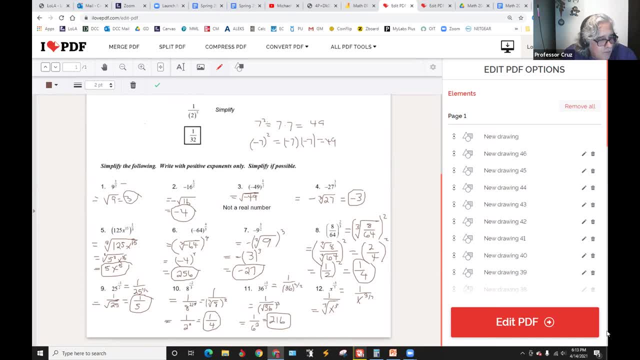 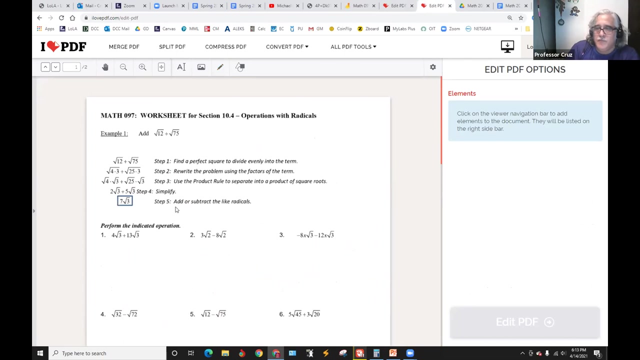 Let's see. So now We're going to move on. We're going to Operations with radicals. Now, I'm sure most people remember that when we were dealing with variables, we had something called like terms. In other words, if you had 2x plus 5x, 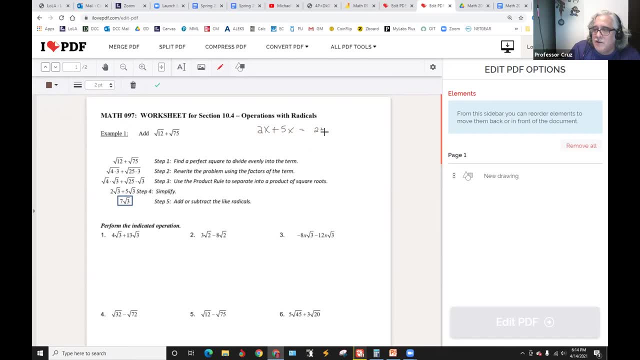 That's 2 plus 5x, You add. If the variables are the same, you just add up the numbers in front of them. It doesn't always have to be positive. They can be positive, negative, both negative, All right. 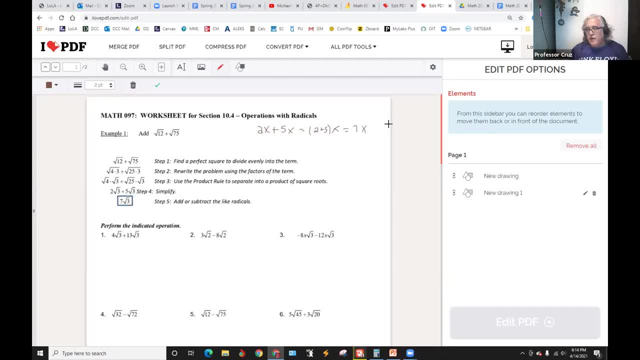 Well, with these radicals, pretty much the same thing can happen as far as adding them and subtracting them, Because If they're alike- in other words, same root, same value inside of the root as well- then we can add and subtract them. 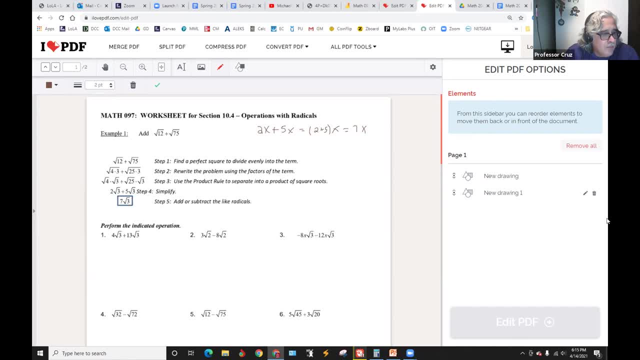 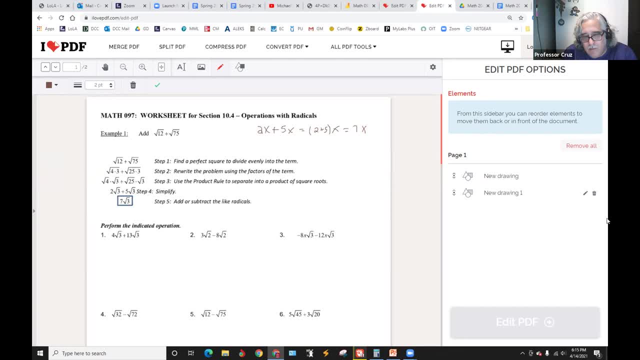 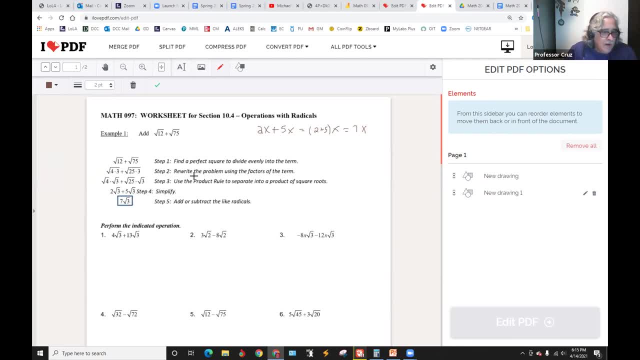 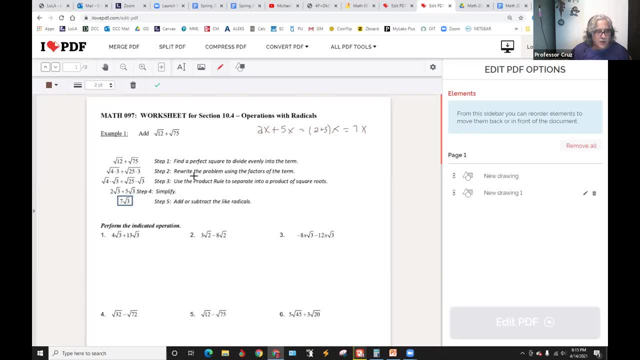 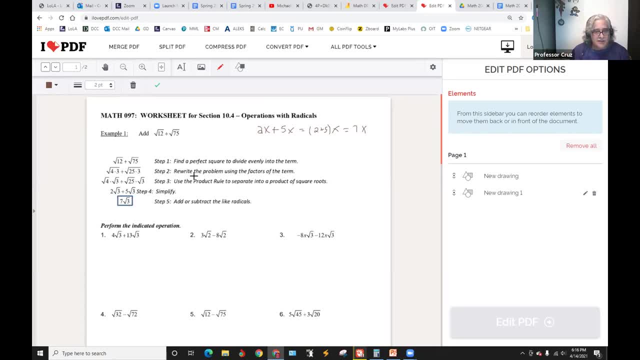 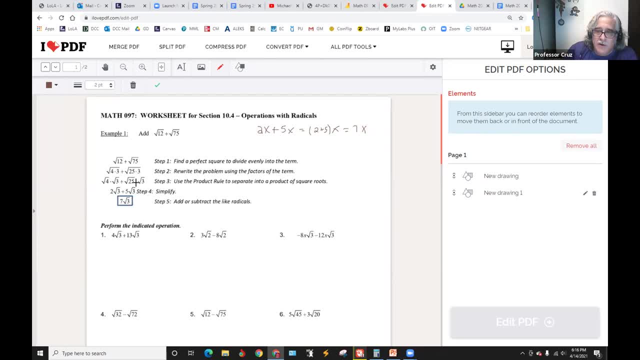 75 is 25 times 3.. Okay, Now, sometimes when you have a small one like this, that's a good place to start, because there's obviously only one perfect square inside of there, inside of 12,, and it's 4.. 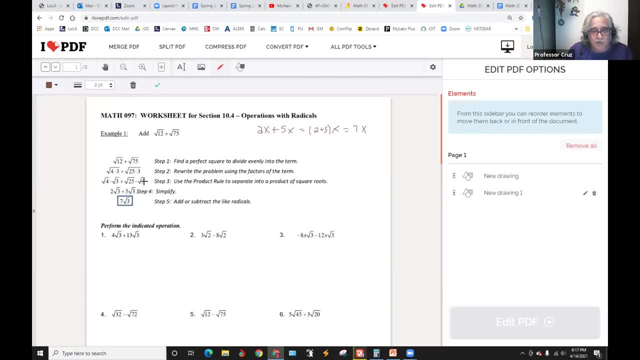 And then you can use the number that comes out. provided that you've simplified it far enough, All right. This number should not have any more perfect squares contained within it. So 3, that factor that goes with 4, to make 12, we can divide that into 75 and see that we got 25,, which is another perfect square. 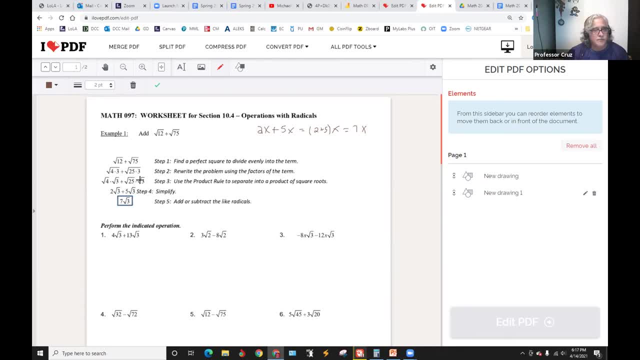 So 75 can be written as 25 times 3.. All right, So now we break it apart into two separate radicals Square root of 4.. Square root of 4 times square root of 3, plus square root of 25 times square root of 3.. 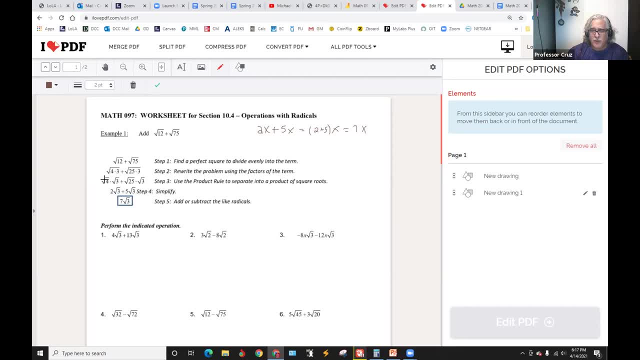 And then these two are multiplied, so square root of 4 becomes 2.. Bring that down, so that's 2 square roots of 3, or 2 times square roots of 3.. Plus 25 times the square root of 3.. 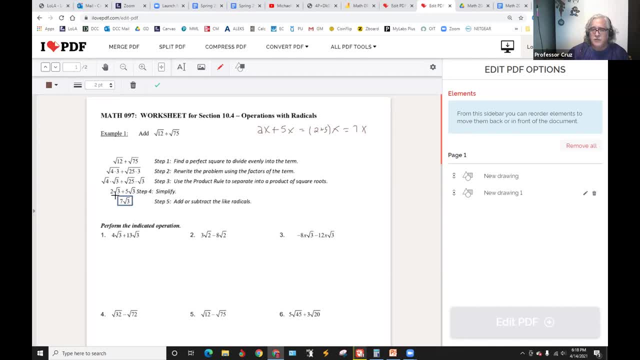 Square root of 25 is 5 square roots of 3.. So now these match. We got 2 square roots of 3 plus 5 square roots of 3.. We've got apples and apples. We've got 2 boxes of apples and then 3 boxes, 5 boxes of apples. 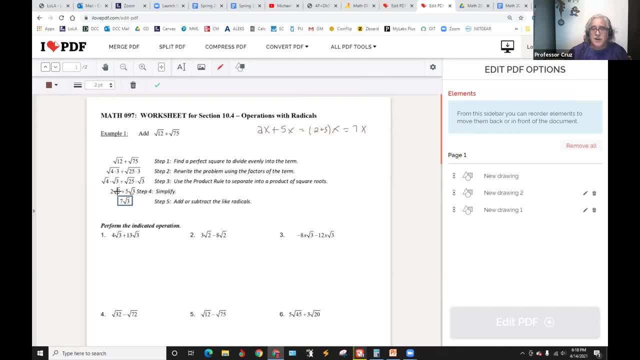 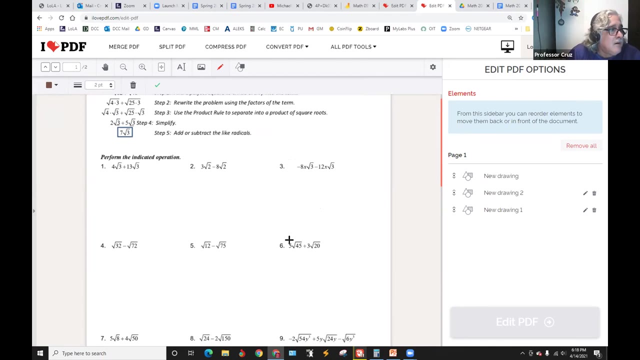 We put it together, we got 7 of them. They're the same unit now, Just like like terms in a sense. So 2 plus 5 is 7.. All right, I'll tell you what. Let's take a break a little bit early here. 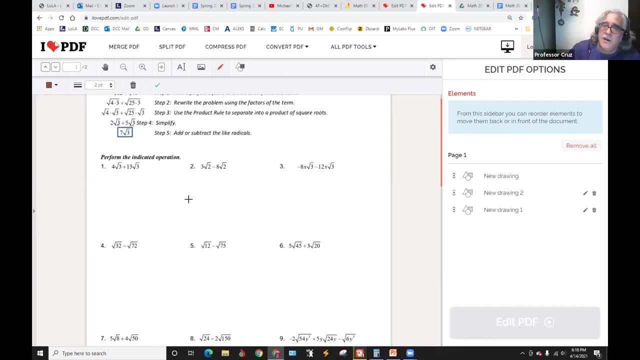 I need to get some air And then we'll come back in it, Because we need to get through this. at least This is for next time, So I don't want to go too far, So just keep looking if you got any questions. 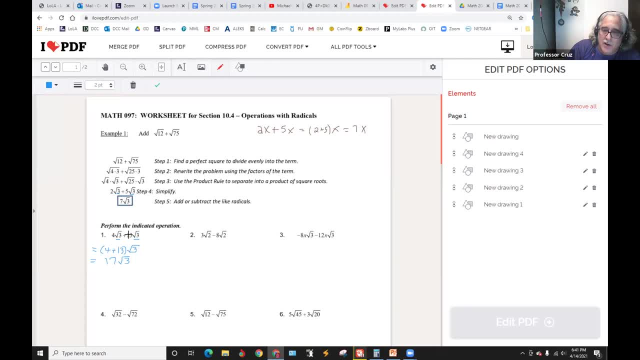 All right. So We got 4 square roots of 3 plus 13 square roots of 3.. Since they're both the same, we can just add the numbers in front: The 4 and the 13. So that's 17 square roots of 3.. 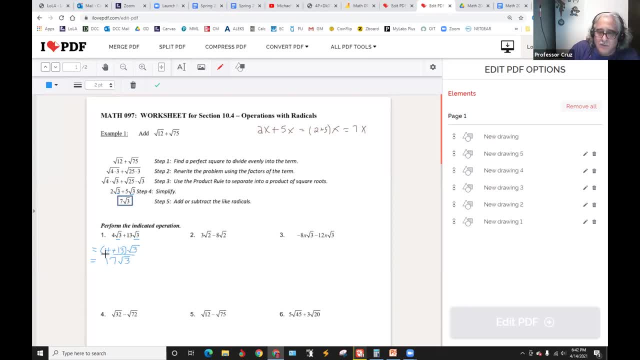 All right, Does that make sense? Yeah, Okay, Now the next one. Matter of fact, the whole First row Are all ones That are That already have a like radical. See this: We got square root 2 and the square root 2.. 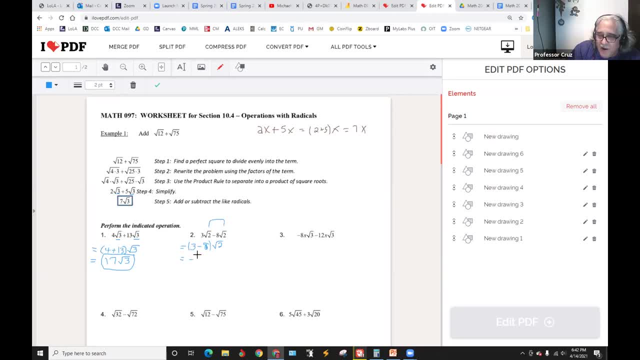 So 3 minus 5, I'm sorry, 3 minus 8 is negative 5.. Square root of 2.. Does that look good? Yes, I got it. Now this next one, 3,. let me just kind of show you. 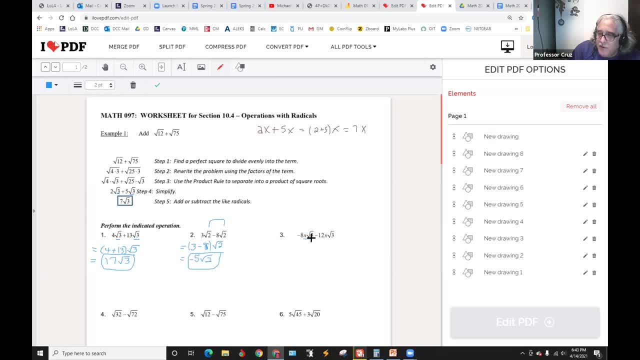 I'm going to give you some of these to work on your own. All right, There we're not including just the root, but also the x, So this is negative 8 minus 12.. And the like part is the x square root of 3.. 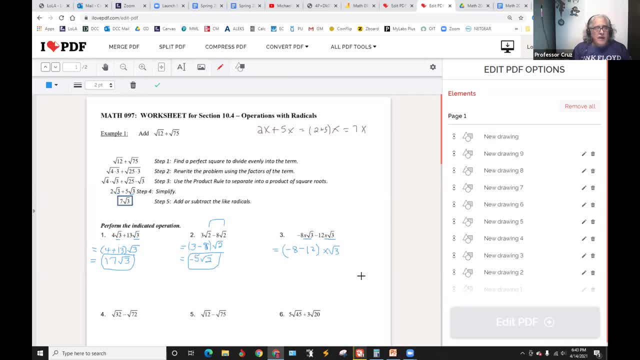 So that variable in front, Well, it's acting like a variable, So that means we can add and subtract those as well, Because it's x square root of 3 is the like term. All right, All right, you see that. 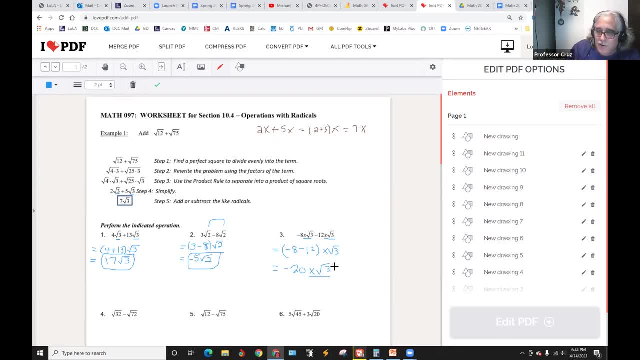 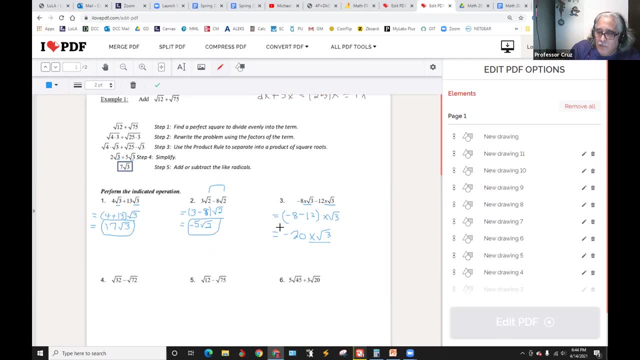 That's the part that's the like term. now It includes the radical square root of 3, but there's also an x in the front. Let's look at this: The x square root of 3.. So this is negative 1 minus 12 x. 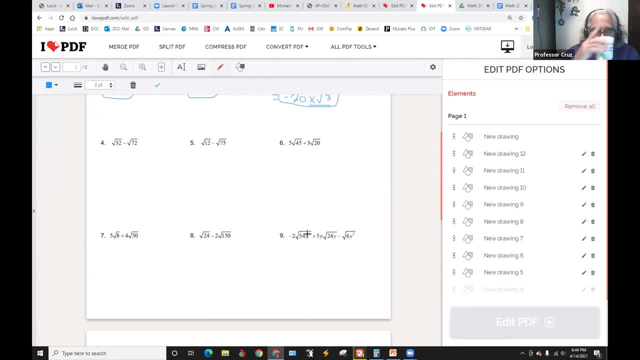 It's negative, 1 minus 9.. That's the like term, That's the right one. So I'm going to have to do the next two things. So negative y minus y, square root of 3.. Negative y is positive y, square root of 3.. 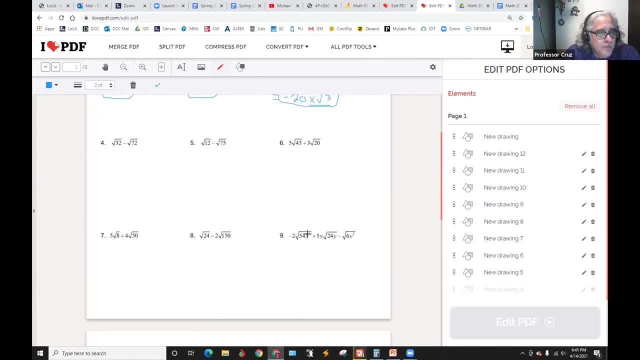 But you have to take into account what that is. Negative y minus y square root of 3 is negative y square root of 3.. Now, this x is negative 2.. Negative x: square root of 3. Why? All right, again, these are not alike. 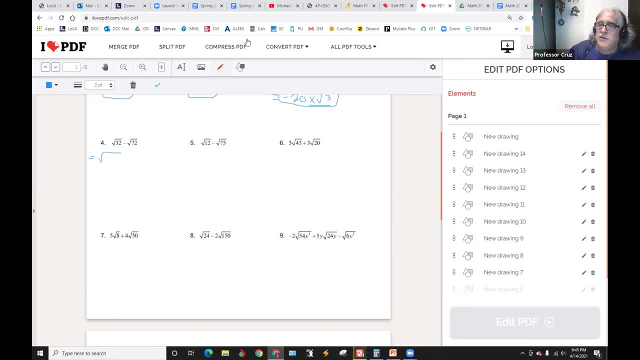 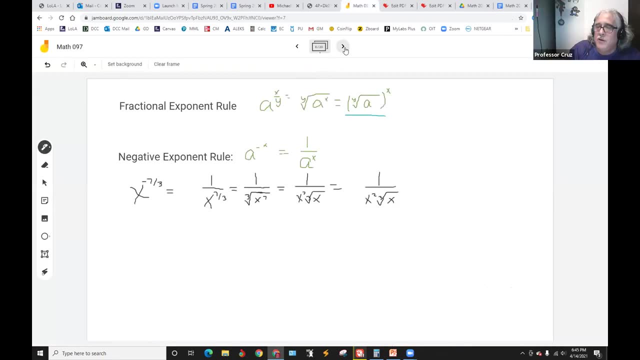 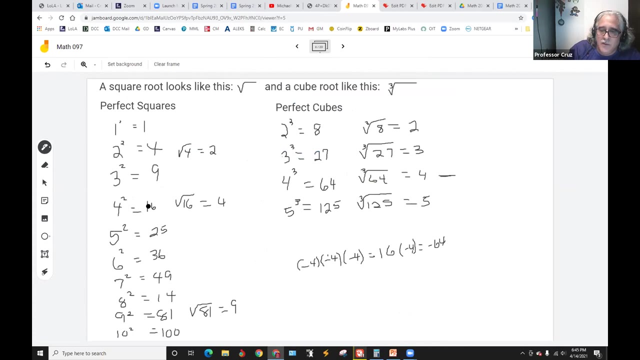 But what can we do to reduce those? Are there any perfect squares inside of 32?? Oh, 16 times 2.. Yeah, I was going to go back over here. See, 16 is the largest one in there. There's no 32.. 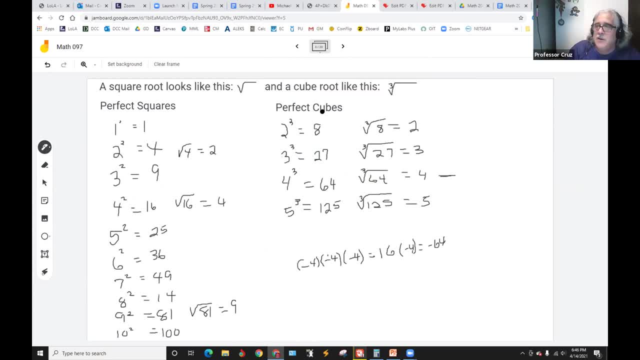 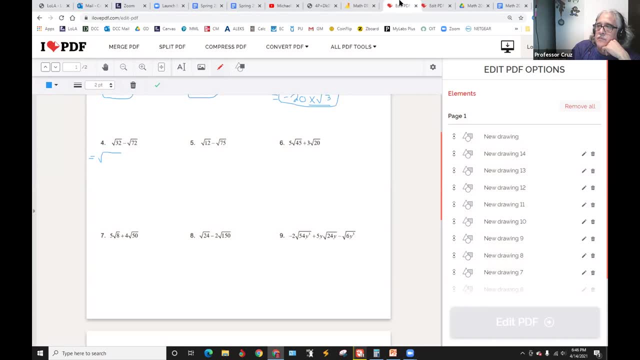 There's 36.. There's 25.. But 16 is the only one that allows us to break it down. So this is 16 times 2. And this is 36 times 2.. Now, as I had said previously, 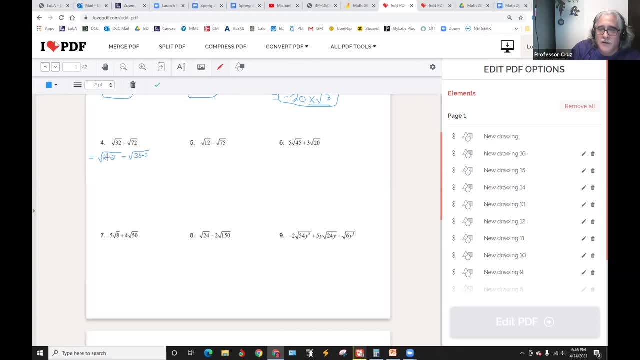 there's supposed to be a multiplication there and there. What, What? Once you get one broken down- and I would recommend starting with the smallest one- once you find out what that other factor is, you can use that to divide into the other one. 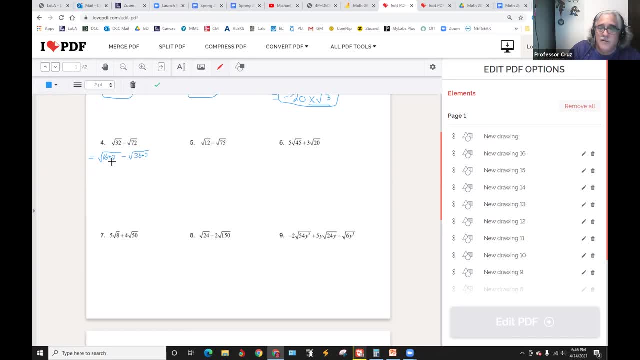 because this is going to be the one that stays in there. So 2 into 72 goes 36.. And 36 times 2 is 72. So we're taking a long like until we understand the problem. So to figure out our way around this, 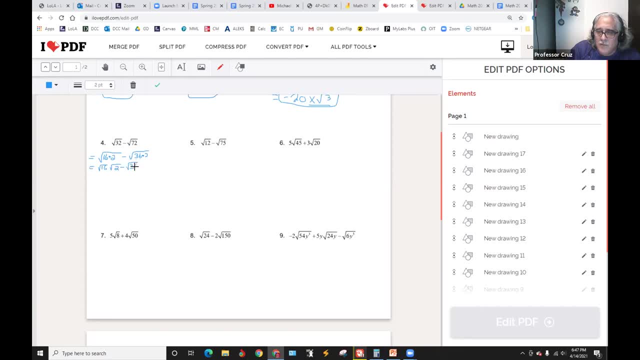 we are going to use the maximizing method Because I know that education has evolved so far. you can just take our math, actually, and you can see that everything is pretty obvious over 60. And the problem is: you're going to be able to solve. 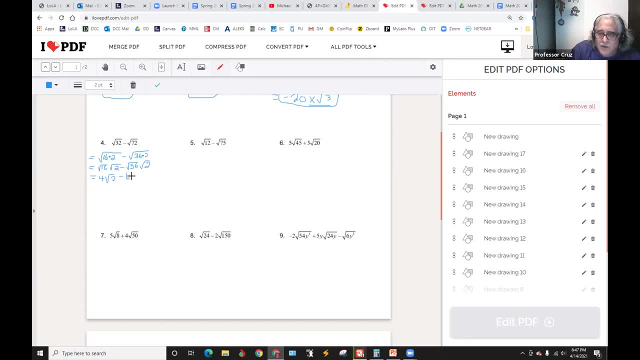 anything in less than four answers And that will just ruined the process. Okay, So a square to 16 is for. Okay, So square to 16 is four. So now we got four minus six square root of two, which is what Negative two. 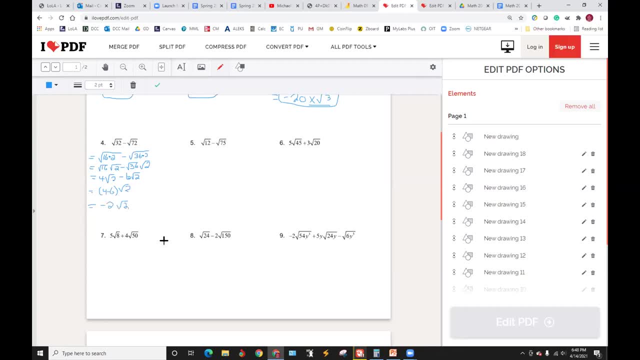 Square root of two Mm-hmm. All right, All right, Excuse me, I'm going to do it over. I'm going to go to my math lab and pull some things out to be able to work on. All right. 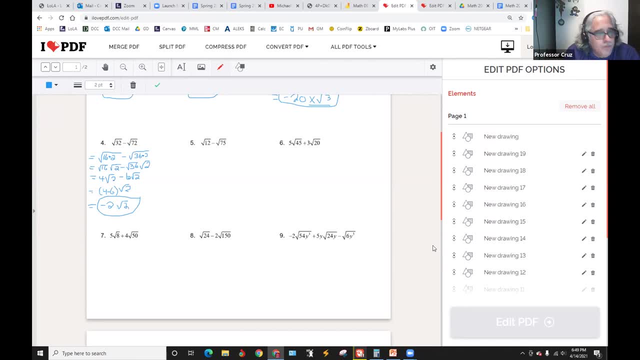 I'm going to go to my math lab and pull some things out to be able to work on, All right, Oh, I know who's going to do something here. I'm thinking about it. Remember the final exam. it's proctored on that proctor- uh, you review thing. so 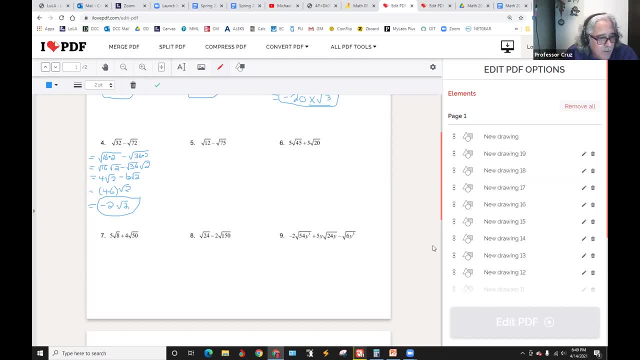 make sure you get that working. i'm going to put it back up there until, uh, last day of class, because you don't really want to go into that cold, because just warning now there is no time at the end of the semester for somebody that forgets to. 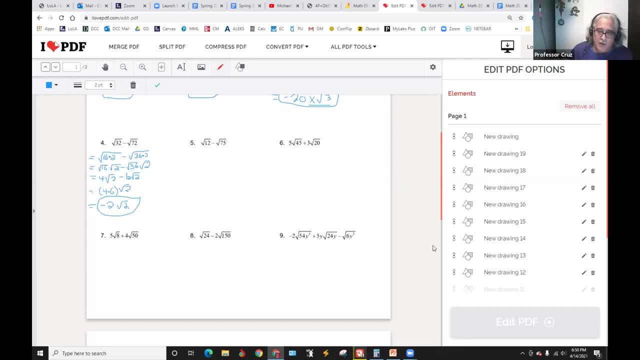 take the exam or they had technical problems the night of the game. i'm going to have it up there for three days, so just remember that. so i'm putting that proctor you review check again there, because i can go in there and see what you've done that kind of thing or not, because 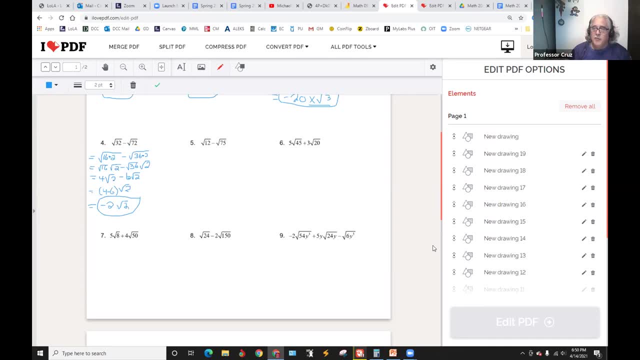 like i said, it's at the end of the semester. i'm under the gun. in fact there's somebody holding a gun to me and want those grades turned down. i gotta do get them done by the end of that first week, by that friday, which is late uh. 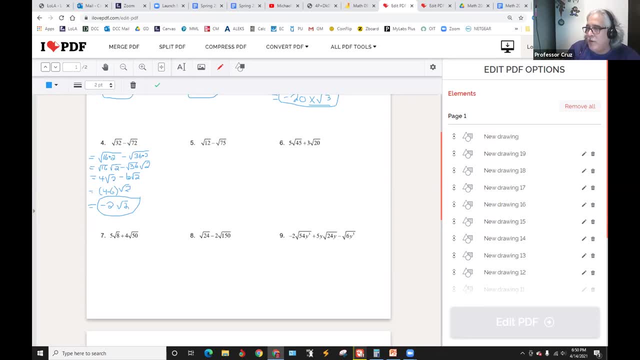 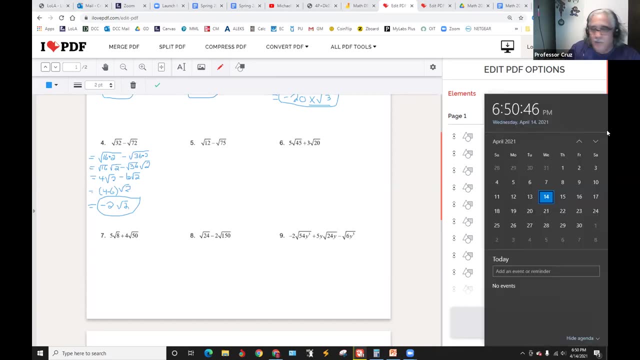 friday of the seventh. so let me bring that all up about the, just so you can see where we're at. we don't have that much time to go, all right, so here's one more week here: 19th and the 21st, 26th and the 28th- the last test is taken. 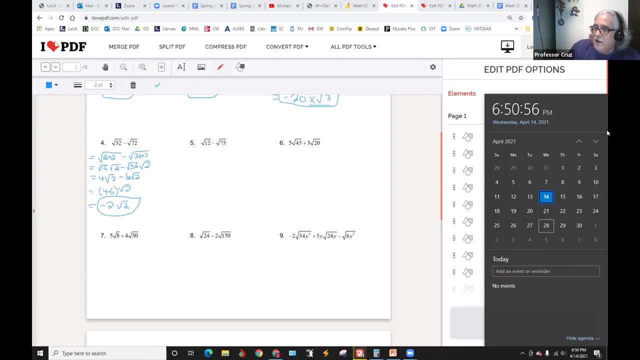 here by this time. now the kind of the problem is, which i don't like, but i can't really figure out a way to test it. um, unless we speed up a little bit, is that when we come back on this day, which is the last day of 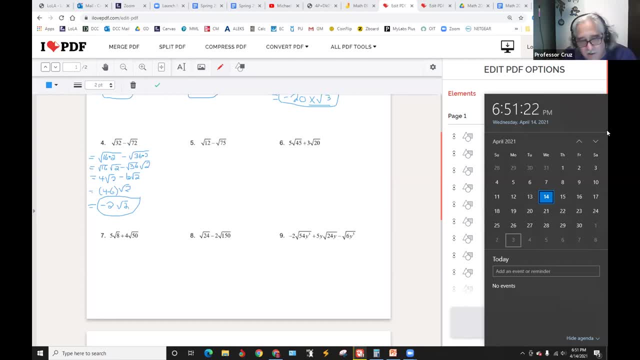 class the third day. that only gives us that one day to uh, to review for the exam now in this class. i kind of think that'll be plenty because we got double. you know, we got two hours and something with a normal class where it just meets an hour, a little over an hour. 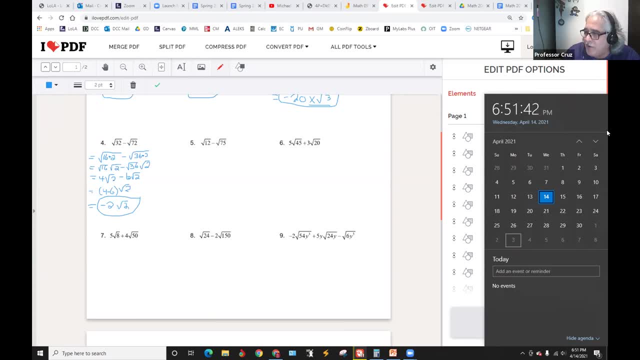 it's not really enough time, so that may well work out all right for this class. i got a tuesday, thursday class which i'm really worried about, more worried about, so just look at that like two weeks we're essentially done, except for the exam and that exam. probably what i'll do is i'll have it third, fourth and fifth. 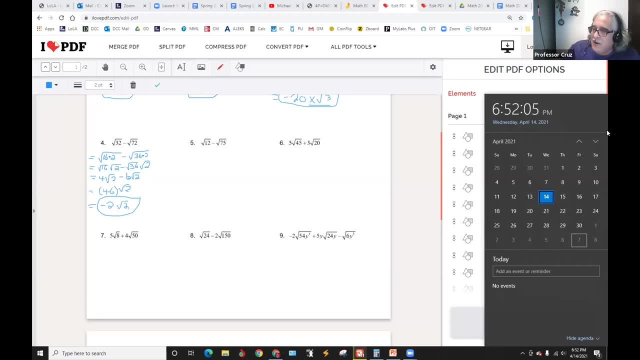 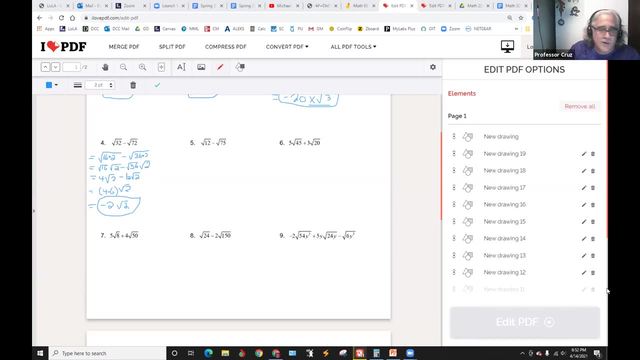 i might be able to do it under six because, like i said this, i got a deadline on friday to get grades done, and so that's a little bit of a problem, but one way to get that done. i'll go to the next slide. all right, so make sure you understand that. if you like said it is: if for some reason you 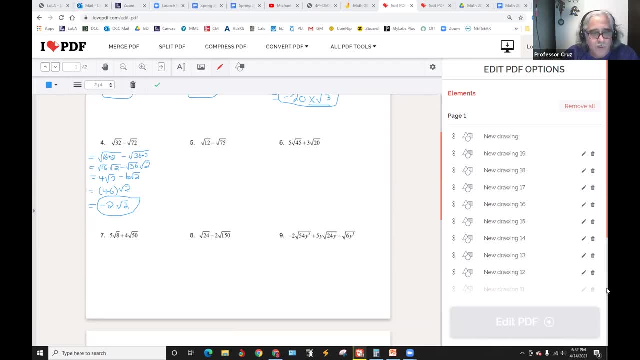 still haven't got that private to you. i'll work and make sure you got it working, because i put that little um proctored review quiz thing out there. it's solely to make sure you've got your system working, because you cannot get through this class without that proctored exam. 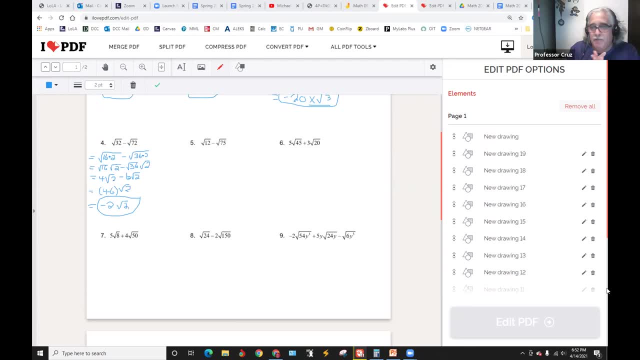 all right. so again now. this one was one that we just worked up there, the two numbers 12 and 75, so we know what to do on that one, but they're not the same, so we got to go ahead. and then the three goes in: 75, 25 times. 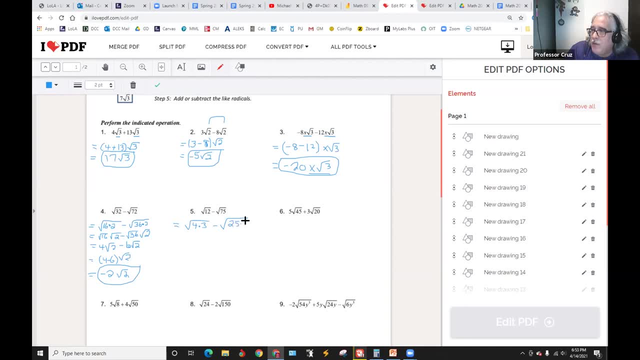 all right, see there, we got a one that that are going to be the same when we finish this. all right, so this one is four, square root of square root of four, square root of three. so that's two, that's the two and that one is five. 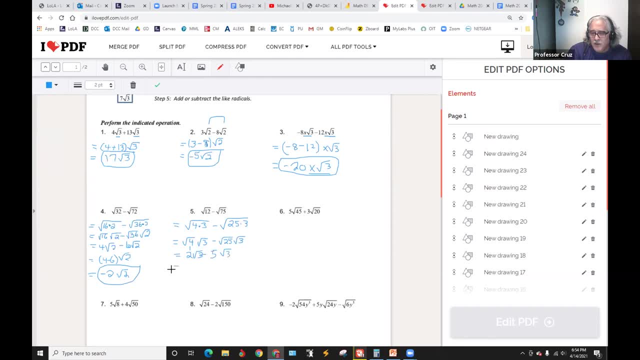 square root of six to it. so, as I said, you can put this in here to see what's going on. two minus five screws. okay, does that make sense? you see any problems with that? that's what I got. okay, usually two would be a good sign. as long as they did it independently, that's a good sign. 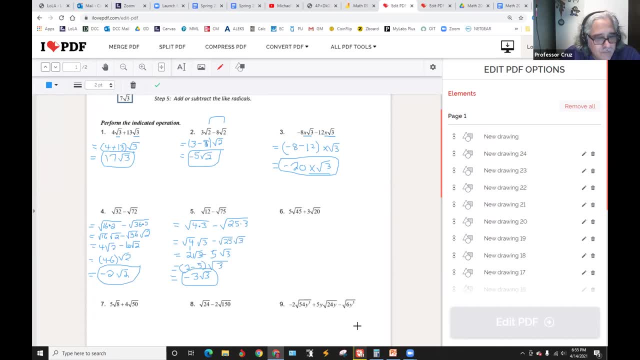 all right. oh, and I was over here looking. I got caught up in that little uh talk about the connect, but I was going to try to find some problems for you folks to work on to after we finish this. that you can. we're going to finish out the class. 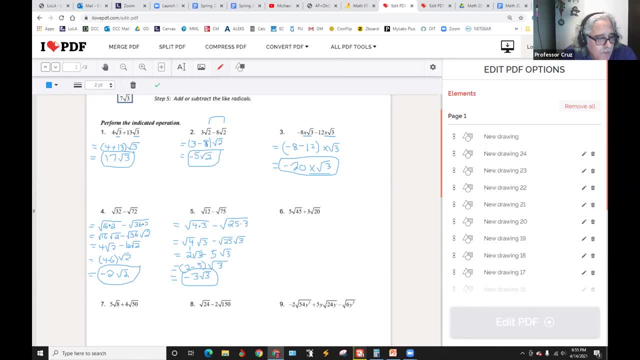 all right. so on this one, all right, we got- uh, I'm going to work on the smaller one, that's four times five, and what's different about this one is that we got a number in front, so anything that comes out is going to have to. does it get added or multiplied? it's going to be multiplied. 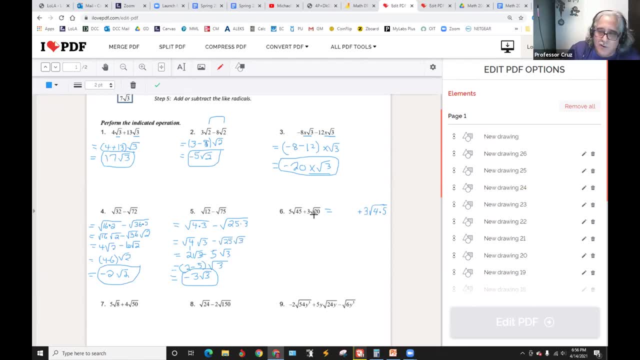 okay, because what this means is it's three square roots of 20.. so whatever square root of 20 is is getting multiplied. so if we can take a perfect square out of there, it's going to multiply that, because that's part of what the square root of 20 is. all right, so now we got a good one here. 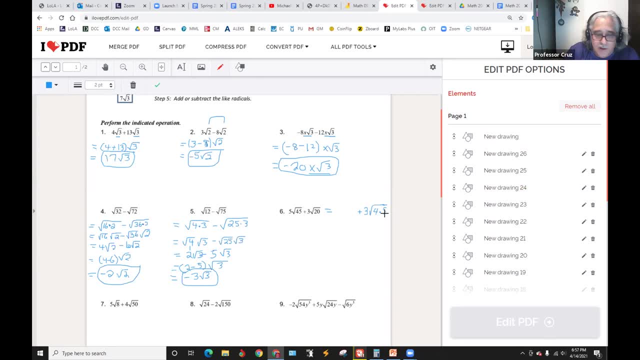 because it's four times five. five is a prime number. we can't reduce that anymore. so use the five into the 45 and that goes nine times, right? yeah, all right. so let me put it in this: break them apart so see, it's five times the square root of nine. 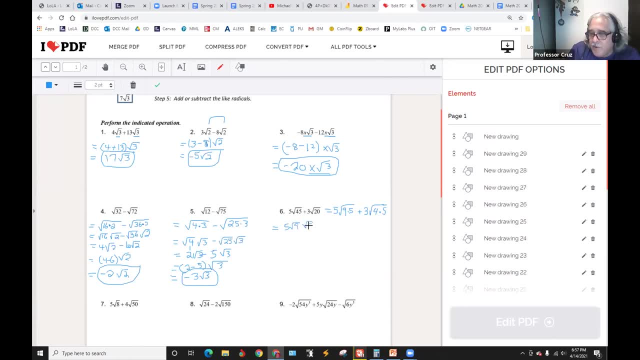 times the square root of five. the square root of five is going to stay in there, so that's five times three. that's the square root of nine is three. the square root of nine is going to stay in there, all right, so let's whittle that down. five times three is fifteen. 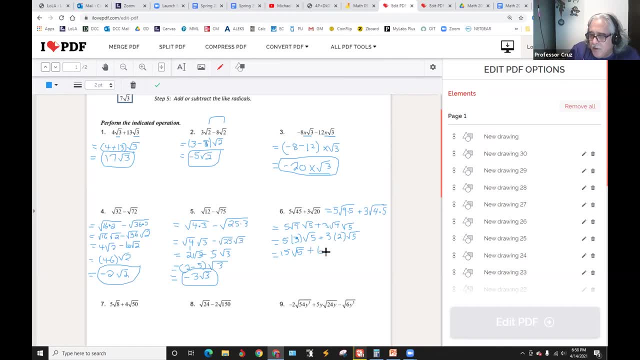 plus six, square root of five plus six. square root of five plus six. square root of five plus six. square root of eight plus six内 plus six over twenty plus six per horse. two and two, then oval, the square root of two. it becomes three, it becomes three. 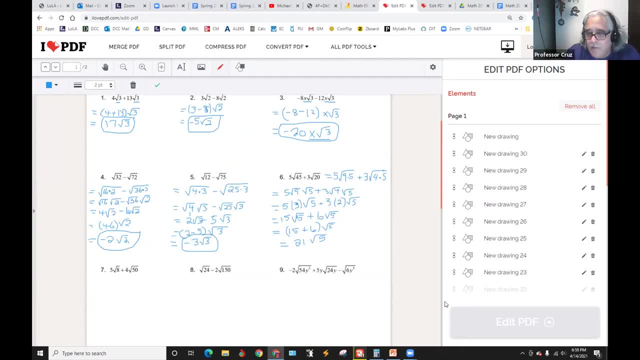 all right, so that, well, and we did it, that's right. next one should be fairly easy, because the screw to 8 breaks down to 4 times 2, and then you can use the 2 into the 50 to give you the other one. i got 30 square root 2.. all right, let's see. 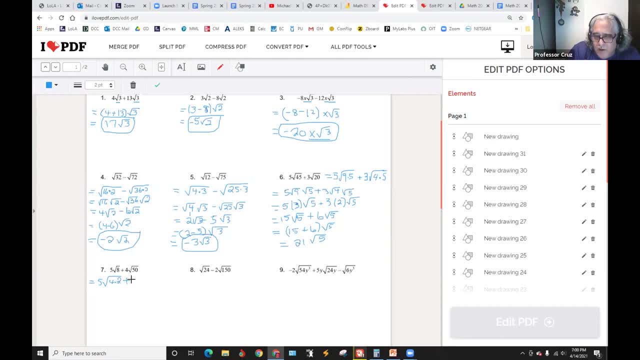 and so we got 4 times 2, so 2 goes into 50, 25 times so, and then this is 4 times 5, So we got 10 square root of 2 and 20 square root of 2, which is 30 square root of 2.. 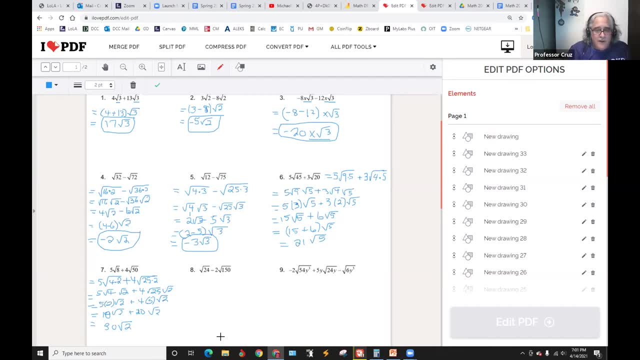 All right, try that next one. Like I said, I'm looking for some problems to show you all the chunking work, But it won't take us maybe 10 minutes to finish the rest of this And we'll do something new we'll do for the rest of the class. 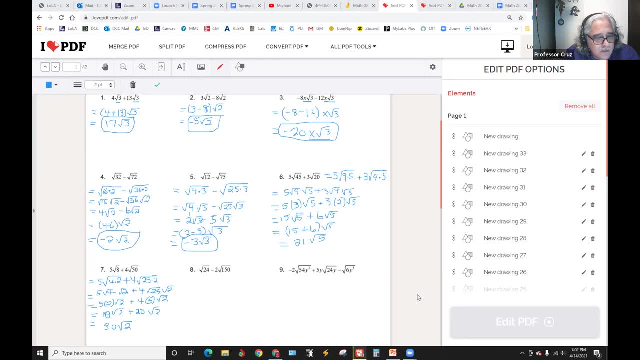 I did some of that And that should be a little broken up and down, But that is what we're going to do. All right, thank you. Thank you very much for watching. I hope you enjoyed it. I'll see you in the next class. 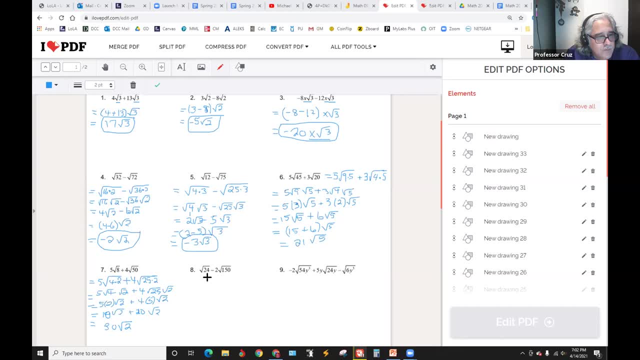 Bye, bye you. No, I don't hear you. Can anybody else hear me? Yes, I do, I do hear you. Did you all finish number 8 yet? 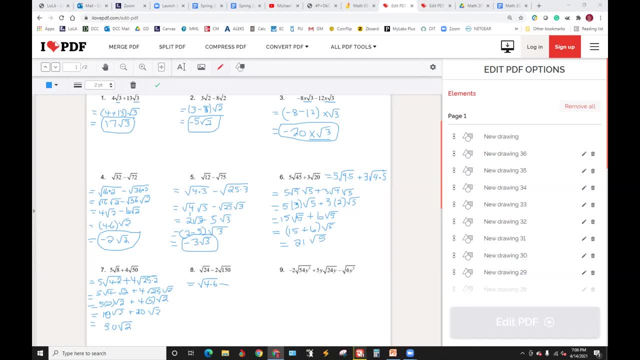 Yes, I got negative 8 square 6.. I got negative 7.. It's worth 3.. Well, it's because I, instead of putting it 4 times 6, I multiply it 8 times 3.. 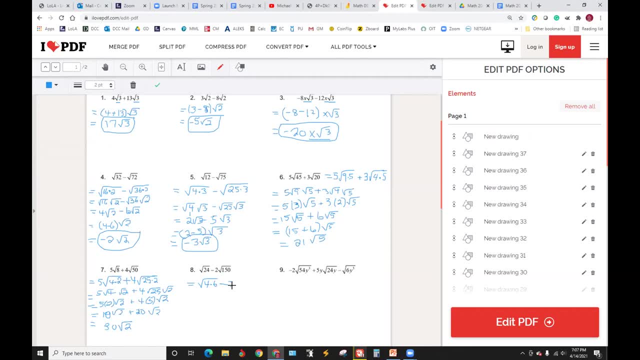 A 50 times 3.. So you multiply it by 6, right, yeah, i did it by six. yeah, i think i just have to remake it. yeah, so the 24 was four times six and the 150 was 25 times six. yeah, and like i said is, you can use that as a hint when you do the smaller. 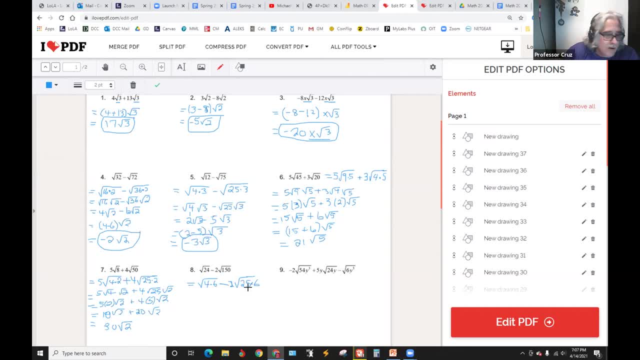 one and then divide six into 150 and you get- if you get back a perfect square, you know you've got it all right. so this is, i'll tell you what this. so this is two square root of six minus two times five square root of six. 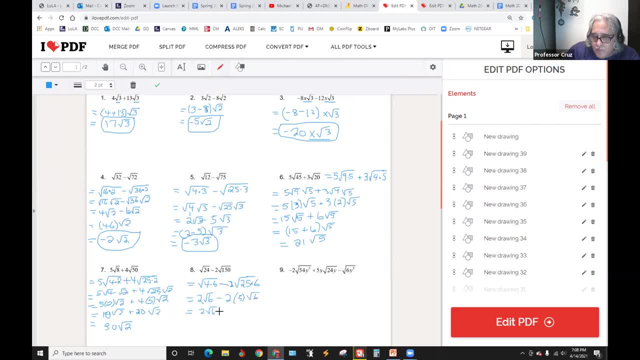 and two minus ten is negative eight square root of six. is that right? that's what i got. all right, okay, all right. now the last one's kind of a mess. it's ends up similar to three. you're gonna have an x come out in front. see if you can do this. and i said i'm trying to. i think i got the answer to. 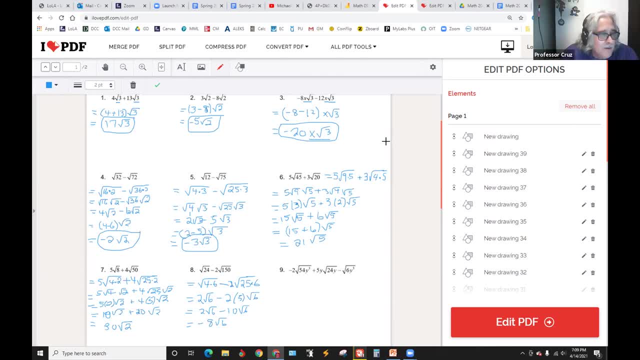 that one you do. yeah, all right, let's see if somebody else can come up with. like i said, i'm trying to find some more to give you all to work. finish out like the last 20 minutes here, let's see. let me look at that one. 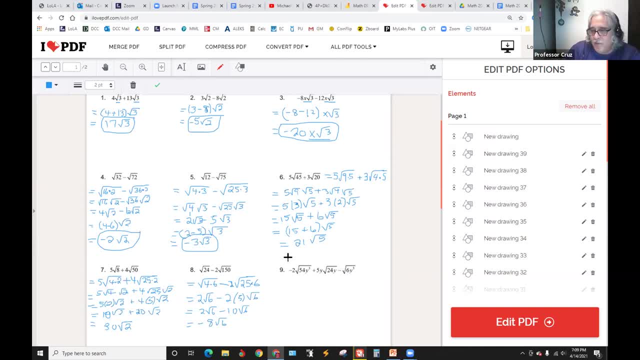 all right, so i'm going to start over here. see that the square root of six six can only be broken down into two times three, neither of which is negative. i can do that one, and then i just finished that one of perfect squares. so six is the number that i need to deal with now. we've got a y cubed in there. 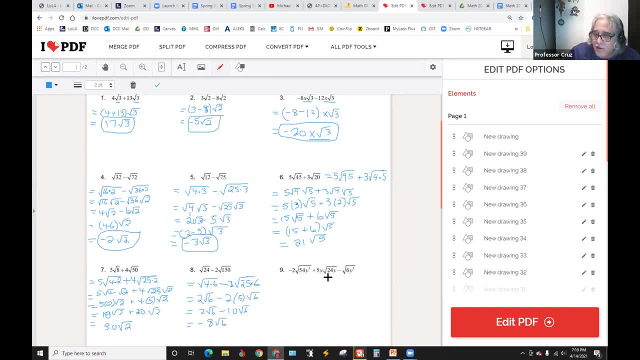 and we can take the square root of that and bring one y out. but what's going to happen here is this: in this middle term, there's a y sitting in there. that's stuck in there because it's smaller than that index of two. so, even if you can't see it, i'm telling you that what's going to be end up staying. 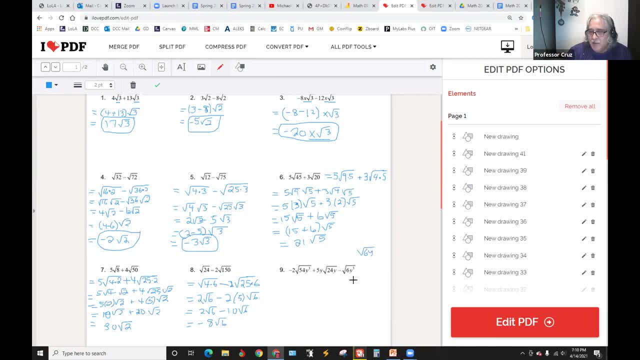 inside is the six and the y. that's why i'm going to use the six to divide into these other ones. all right, so this is going to be six times what. six times six times nine? well, nine times nine is a perfect square, so that's good news. 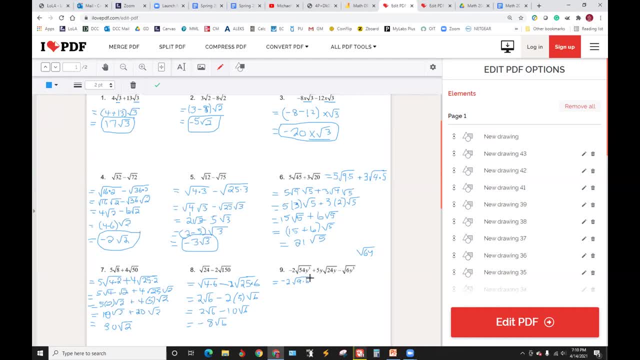 and then there's a y-cubed. we'll deal with that next and six into 24. well, that's the one we did over here. that's four times four times six, and we've still got a y in there. now, if we got any hope of putting these all together, there's. 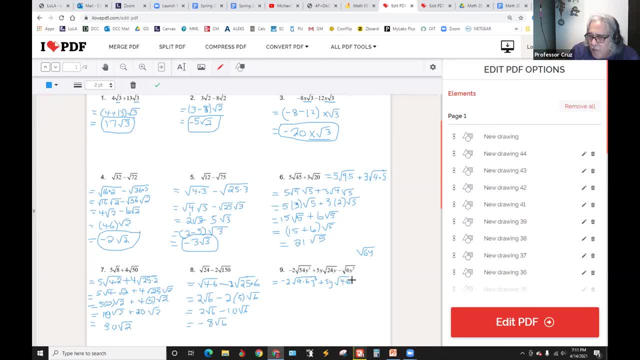 going to be a y left in there, and then we're going to do the same thing we did with the y, and then we're going to do the same thing we did with the y, and then we're going to do the same thing. both the first and the last. both have one y that's going to stay in there, so that's good news. 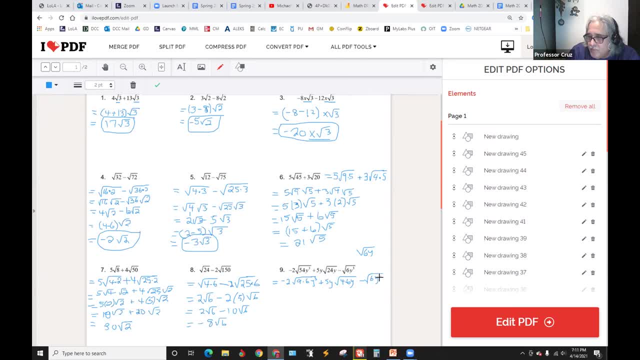 so so, so all right. so this is going to be a square root of nine, and one y is going to come out. square root of nine is three and one y is going to come out and one's going to stay in there, and one's going to come out and one's going to stay in there. 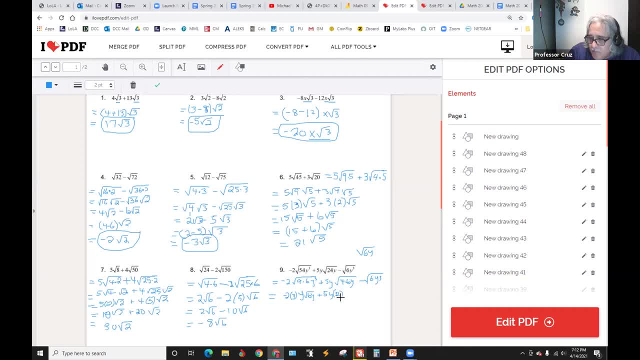 that's going to be two, and then the y is going to come out because there's y cubed. so square root of y squared is going to give us a y out front And then six Ys staying in there. All right, Let me switch to a different color here. 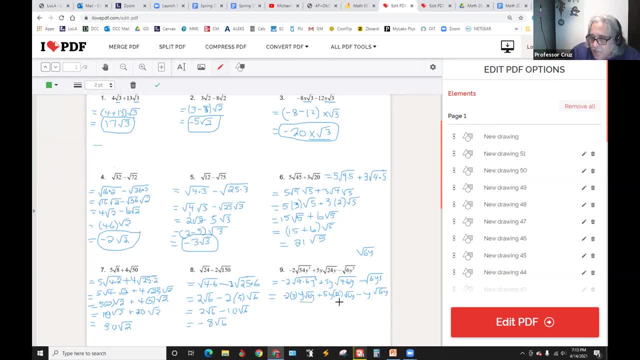 All right, So here's the part. Well, I can't really do it on that one because I got the Y over there. But see, we're not only matching up the six Y, we're matching up the Y that's in front of it. 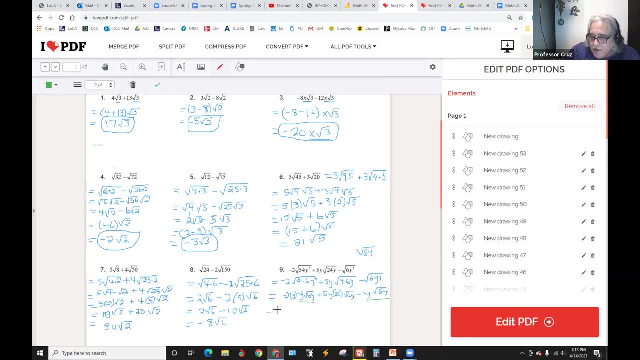 But I'll fix that other one in the middle. So this is negative six Y, square root of six Y. All right, All right. So again, So that's the part that's alike. So what do we have left? We got negative six. 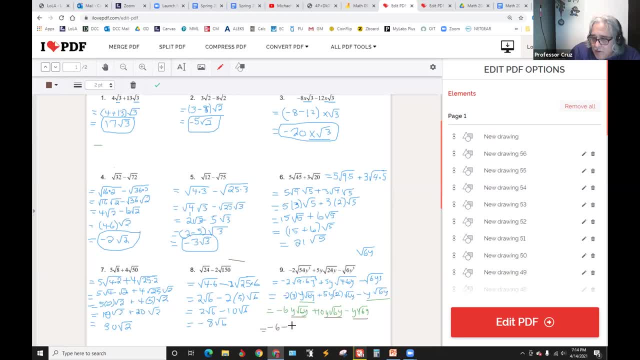 We got plus 10.. And we got a negative one Square root of six Y. So that's a negative seven plus 10 is three positive Y square root of six Y. Does that look good? Yep, That's what I got. 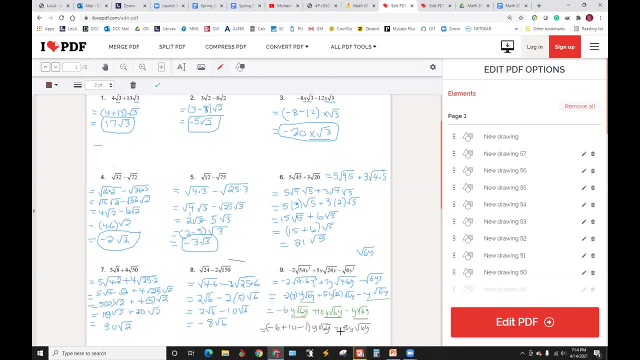 All right, Same here. All right. So what I'm going to do is I'm going to see if I can. Well, I'm going to see if I can screencast this to you and see if you can see it well enough. 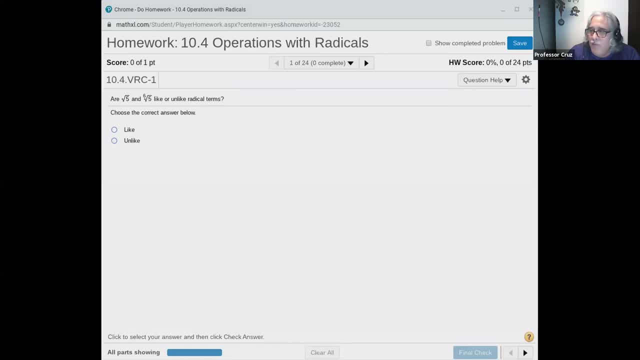 All right, You can see that it looks like All right. So tell me, Are these like terms? Yes, They are. I would say no, Because the second one is what? Sixth root, And this is a square root, right? 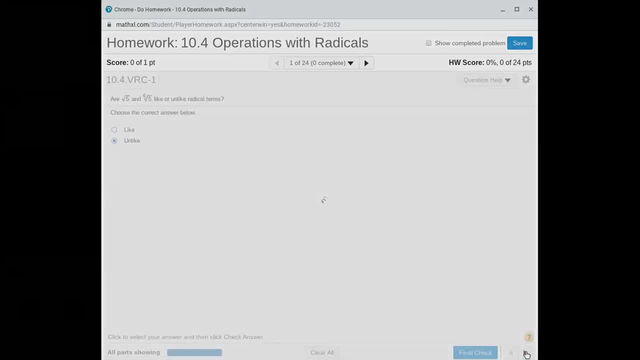 Yeah, So these are unlike, All right. All right, Are these Like terms? Yes, They're both fifth roots And they're both got an A squared times B. They're just in a different order. All right, Are these alike? 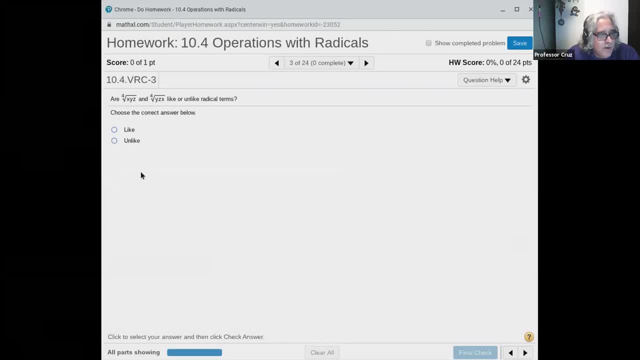 X, Y, Z and Yes, Yeah, They're alike, Okay. Okay, What do you think it's like? Like or unlike? Like I guess Like or unlike, Like, Like I guess technically- What's like about them? 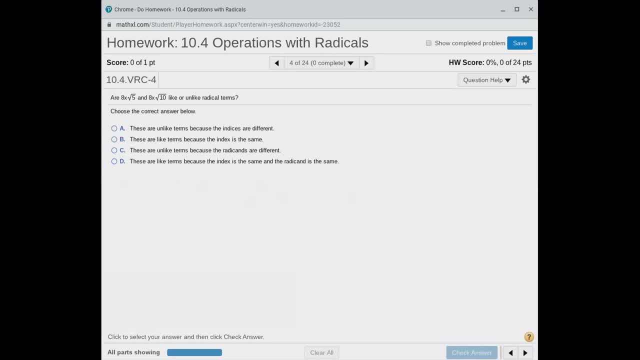 They're both. They both going to be multiply. Well, I mean, I'm going to remind each one of the radical- Yeah, that part's the same, but the radical part. Yeah, that part's the same, but the radical part. 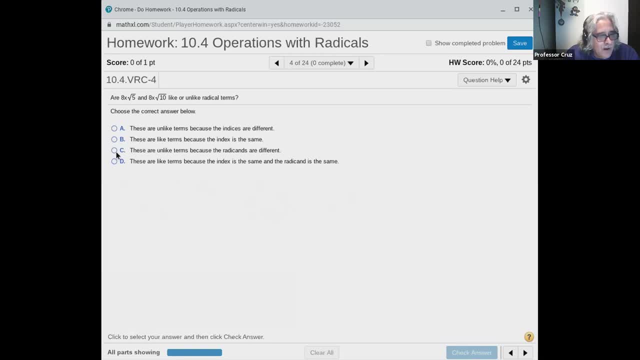 It became like a great role. What's inside each one? What's that thing? Yeah Well, I don't know. I don't know. I mean, if we multiply two times, I mean two times five. What is the like term? 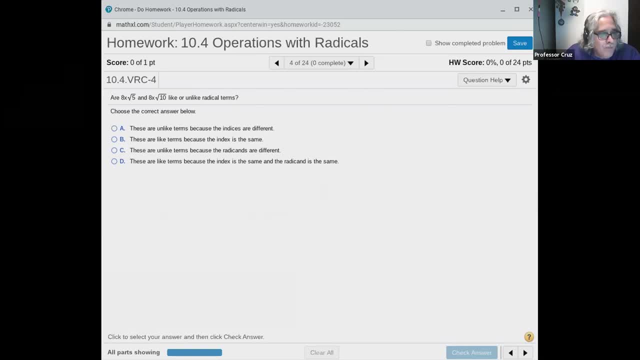 What is the like radical then? What is it? What's the like radical? You should be able to tell me that if they're both alike, Which one is alike? Square root of five or square root of ten? Square root of five. 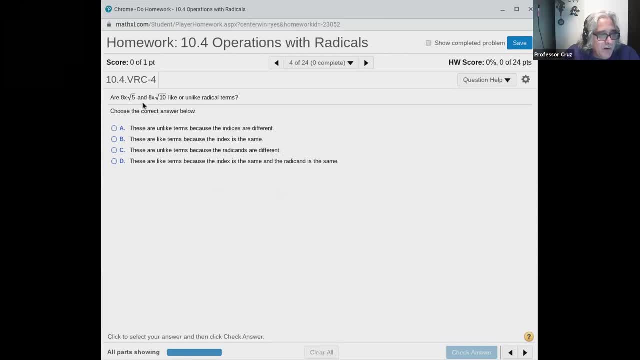 I'm confused. Are they both the same? Let me ask that again: Square root of five and square root of ten? Square root of five, I guess? Okay, So you're saying the square root of five is like to what? Where's the other one like it? 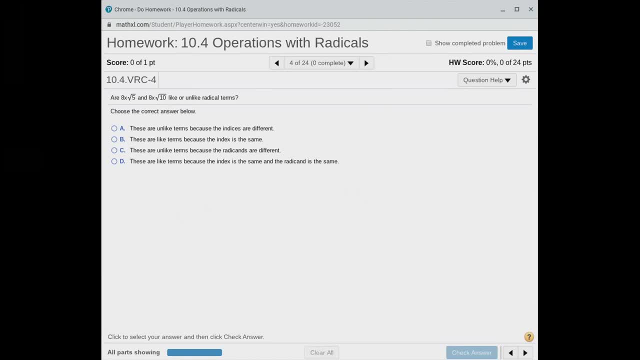 I mean in my mind I'm seeing it like this, For example, what you did with that six Y. You just take it and you remind the same. Well, but that's only part of it. okay, That part is the same, yeah. 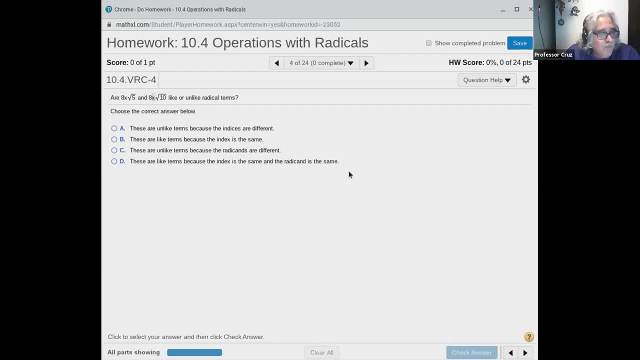 But I'm talking about the rest. What's the radical part? Oh yeah, I don't know. See, that's a square root of five and this is a square root of Ten. I mean, you're right, So they're alike. 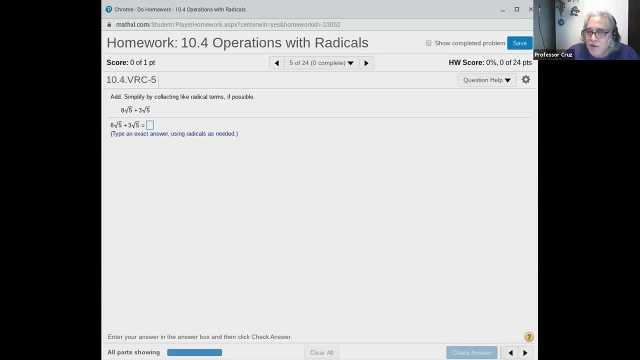 All right, So see if you can work this one out. This one should be pretty easy. Wish I could write on here: 11 is square root of five. Yeah, Plus three is 11.. Yes, Yes, 13 is square root of three. 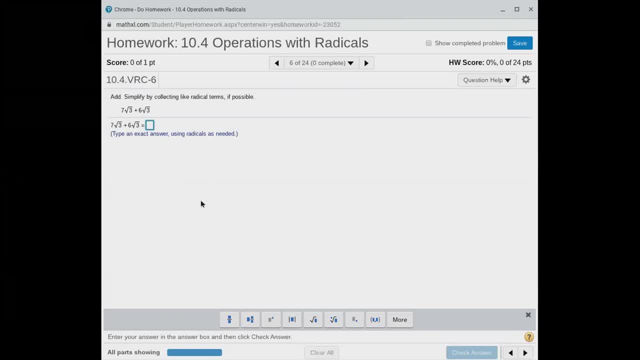 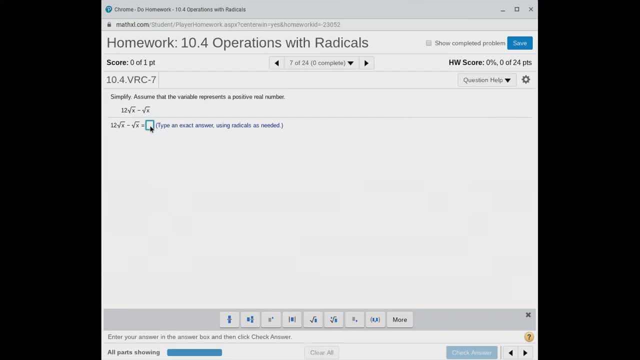 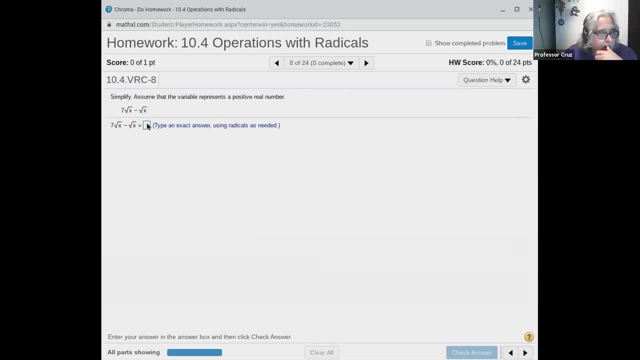 Six, a square root of five, Yeah, seven, take away one. Eight square roots of three and three square roots of three. Oh, B, seven. I mean nine, oh yeah, because they're adding nine squares Okay. 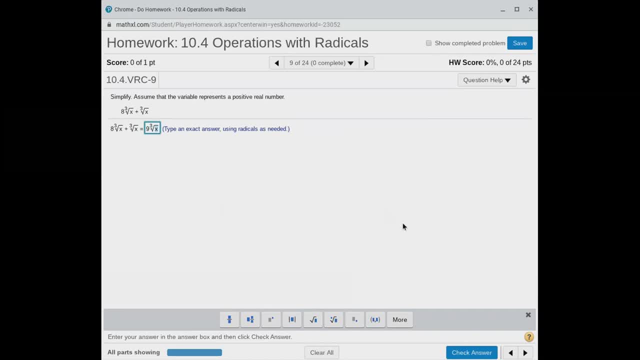 Okay, Eight plus one. All right, these ones have got to be simplified, so. So what happens with that one? That's more like what we've been doing here, So we have to break down the 125.. 125.. 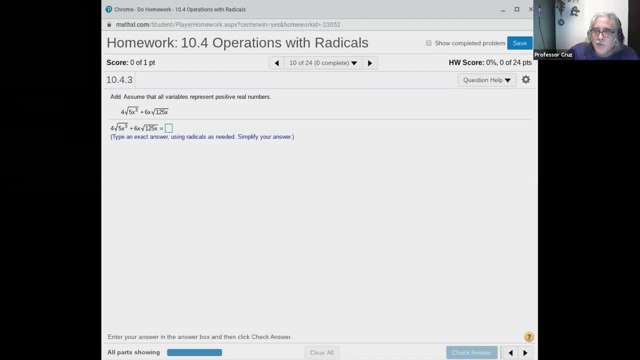 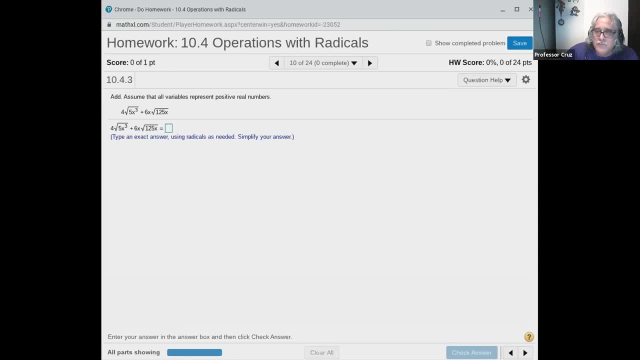 so is it 34 x 5 x square 5x, yeah, 34 x square root of 5x. so so 9 times 3 minus 2, 9 times 2, and then, uh, oops boy, am i getting tired, or is this one just not gonna do? 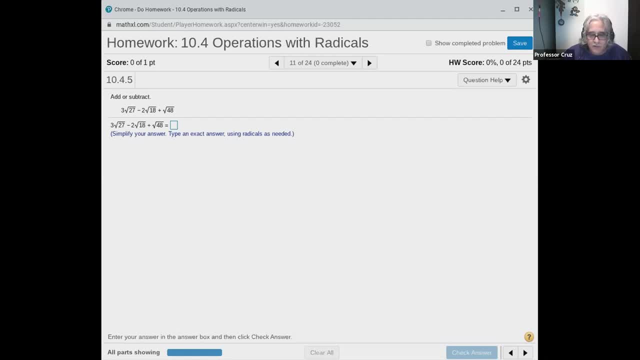 completely together. so did you? so did you? uh, let's see to you, to you to, yeah, All right, See, that's why I was just about to ask, Because if they all don't have the same matching, what is it? whatever, then it still ends up just being a problem, right. 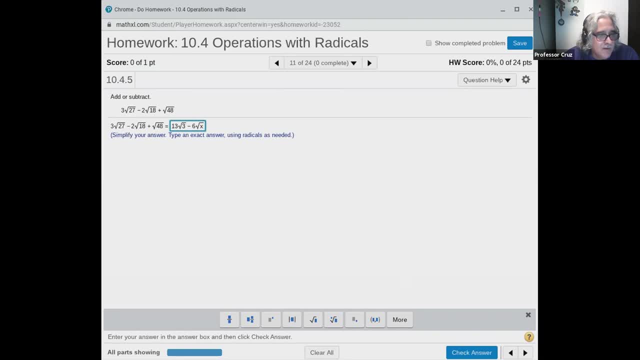 Well, I mean, I've seen them like that before. It's just that we didn't have anything like that on the worksheet. All right, But that's not unusual. They're just going over basics in the worksheet. So six is three to two. 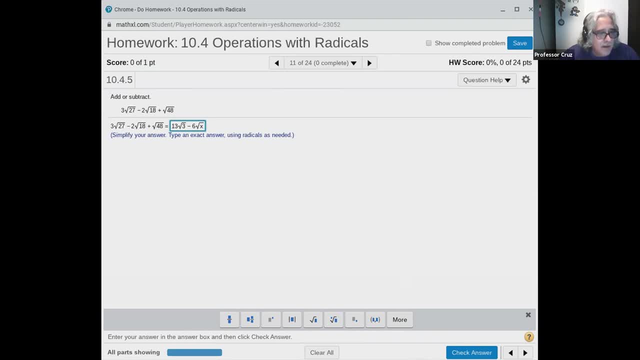 So nine and four is 13.. Not X. What do I got? X and Y is two. X and Y is two. So we got to think cube roots now, like eight, 27,, 27 is too big, So look for eight as a factor of 24.. 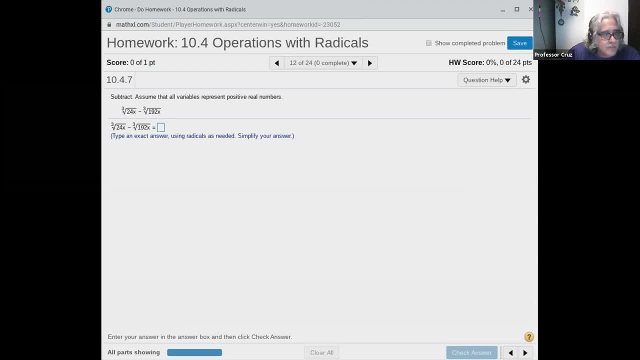 And then use the remainder thing, the one that stays in there, as a hint for 192.. Because the 192 is large, All right. So this is 24.. It's four times, I mean eight times three, So it looks like three. X is going to stay in there. 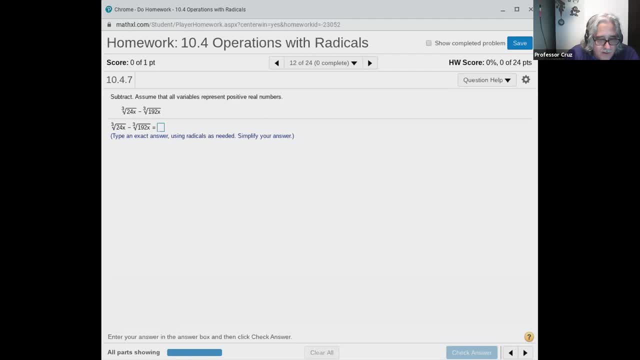 So let's multiply three into 192.. What do we get? 64.. 64.. So that's a good one, because that's a perfect square, All right. So we got Square cube root of eight, which is two, And then three X stays inside. 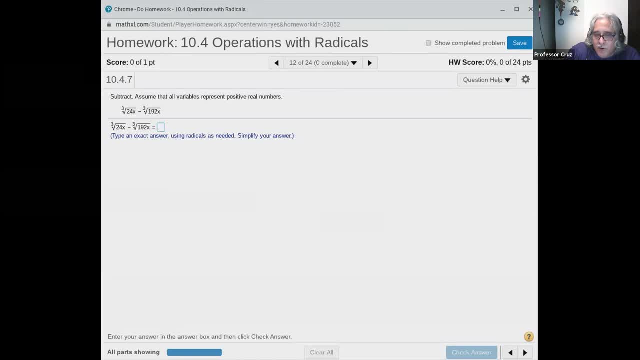 We got the cube root of 64, which is four Takes on that negative sign, And then cube root of three X. So that's two minus four. Thank you, Let's see. Okay, let's write a square. So it was two. 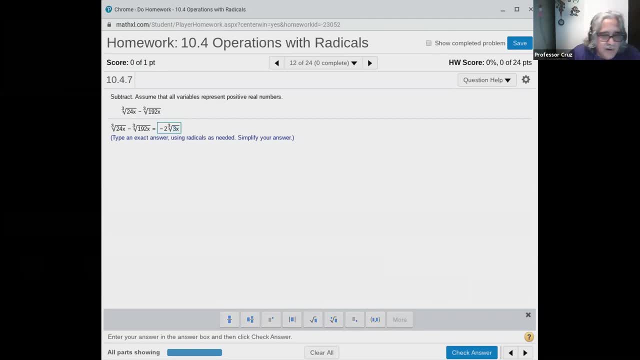 And then three X, And then four X equals zero. 1. 1., 2., 1., 2., 2., 3., 2., 3., 4., 4., 5., 7.. 8., 9., 10., 11., 12., 11., 12., 17., 13., 14., 15., 14., 15., 16., 17., 18., 19.. 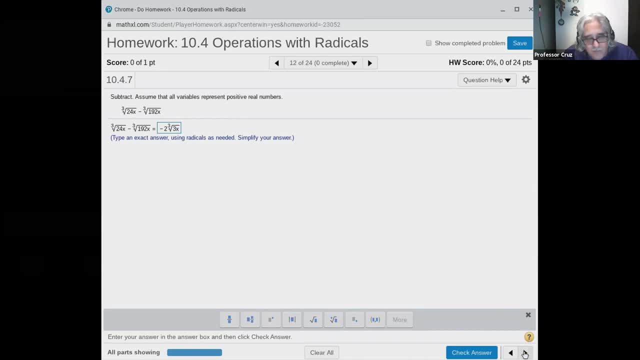 20., 22., 25., 23., 24., 26., 27., 28., 37., 29., 28., 29., 30., 31. 32.. Yeah, Well, I was trying to tell you the trick here is okay, find your perfect square in 24.. 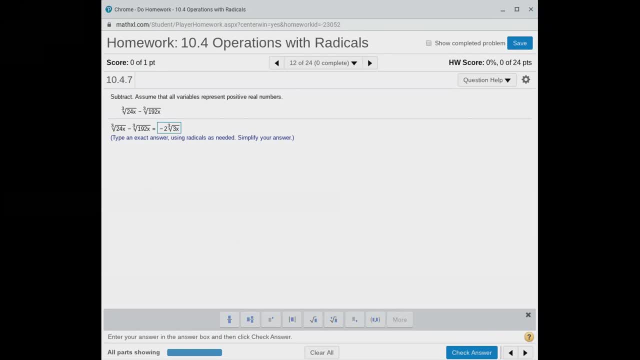 There's only one of them that's going to work. It's 4 times 6.. Then use the – I'm sorry, 8 times 3.. It's cubic root, So use your 3 into the 192.. Like I said, use those stamps. 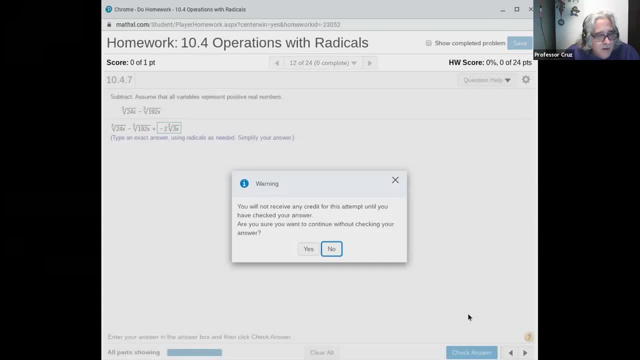 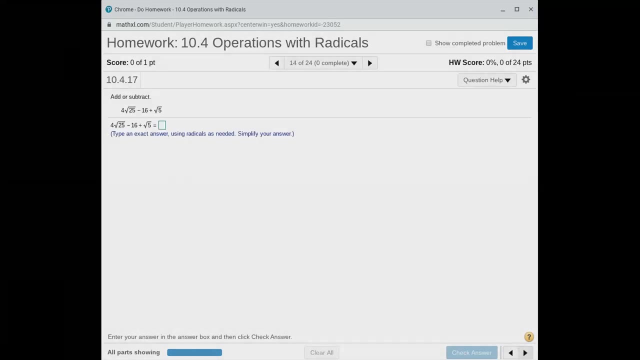 Let's just do one more. Let's just see. I don't know if I want to do anything. Let's see This one Or this one. Try this one. This is not too bad actually. I'm looking at one of that little board. 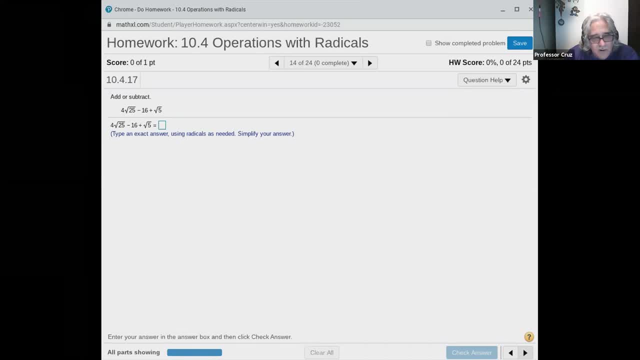 You just can't see it because it's on my – it's not on the share, But I'll let you see them when I'm done here. Is that 14 square root 5?? I see Now you're working too fast here. 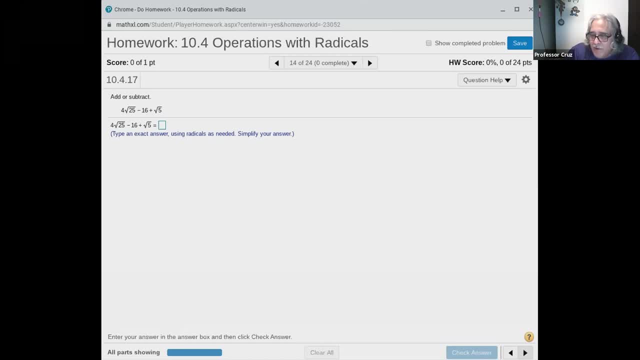 So 4 times, the square root of 25 is 5.. That's going to be 20.. Okay Now, now you do this one more, One square root is going to – left is going to be the 5.. So that's 20 minus 16.. 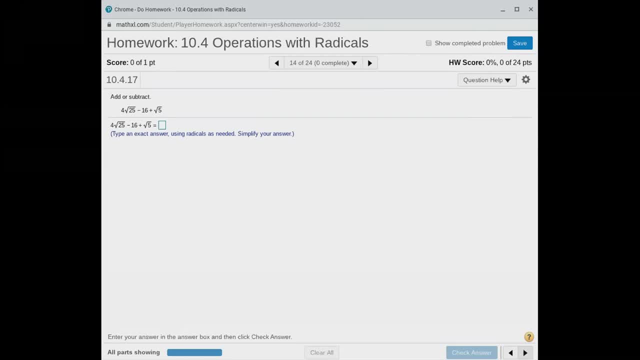 So that's 4 square – So 4 plus the square root of 5.. Alright, I saw the square root. Alright, Right, Nothing happened with the 5.. The square root of 5 just stayed on its own. The other two ended up being the same. 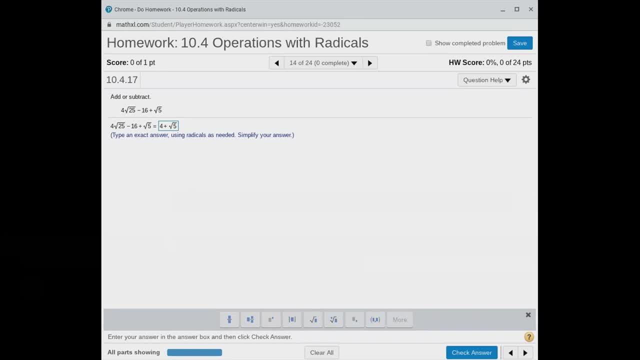 Okay, so just real quick. so when you end up to where you can't add them together, and then it is 4 plus square root, 5? Yeah, because they're different terms. 4 is whole numbers. Okay, So here's the work. if you want to see it here. 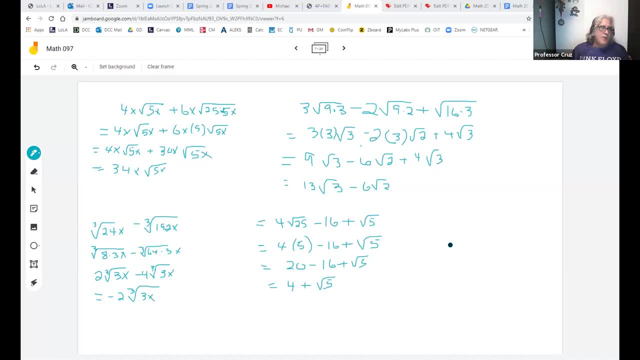 That I was doing on all the ones that weren't broken down. In other words, we didn't have to find the roots. I don't know, are y'all as tired as I am? I don't know why this class is. this class is. 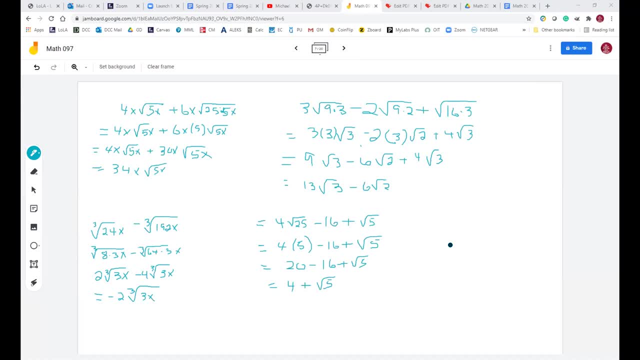 It's the rain I'm talking about for the semester. I don't know, It's late at night. I'm just wondering if I'm going to make it to the end of the semester. I don't know if I'm going to just drop over. 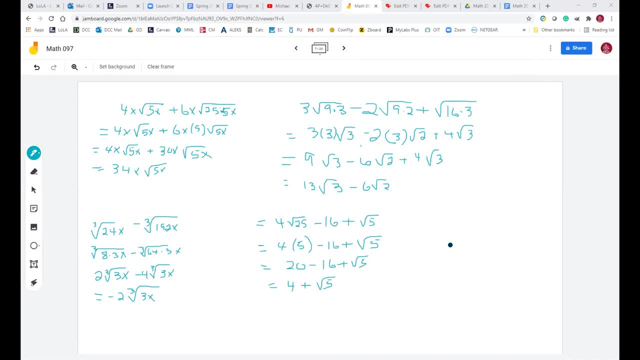 You only have a few more weeks. I know, I've just never been this tired before. You'd think that just working in front of computers and all that would not be as much work as jumping around in front of a classroom. All right, so have as good a weekend as you can. 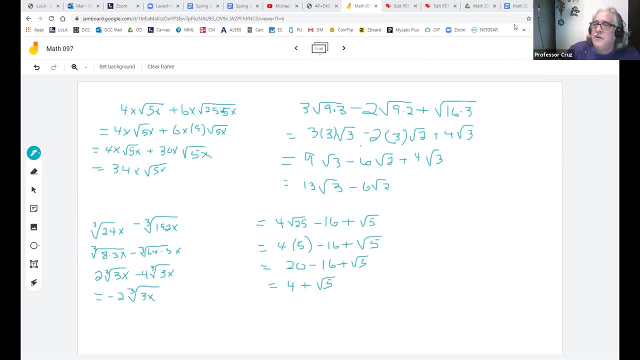 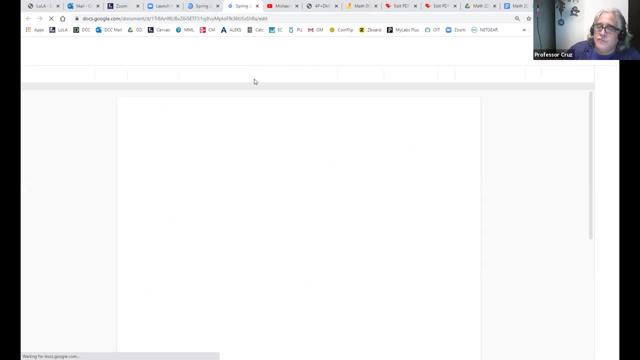 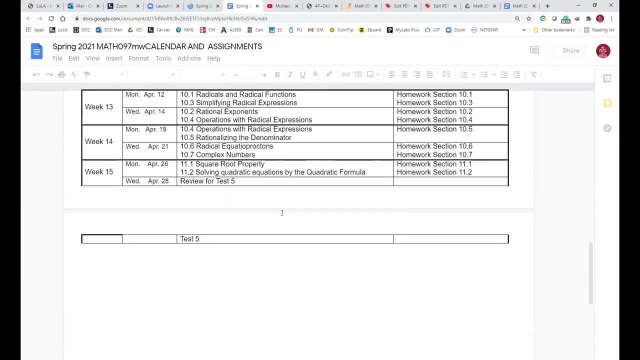 Monday, we will continue our journey. So all right, yeah, next time we got the multiplication, the division, and then we can use multiplication. I'm sorry, it's just multiplication, Rationalizing the denominator. It's sort of like dividing. 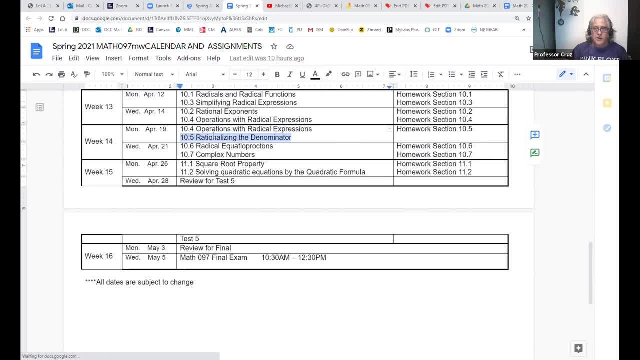 You don't really have a strict operation for dividing with rational numbers, But this thing called rationalizing the denominator essentially does the same thing. So it's remember how division is the multiplication by the reciprocal, It's sort of like that. So we just need to figure out how to multiply.